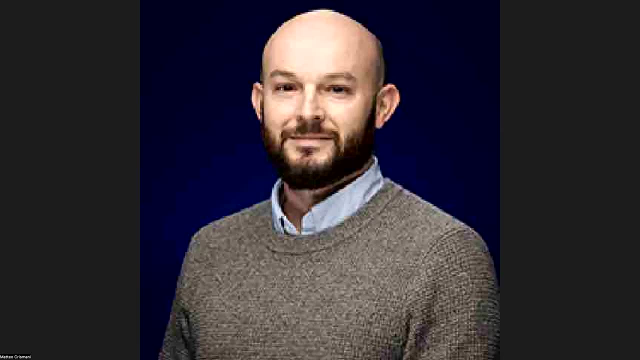 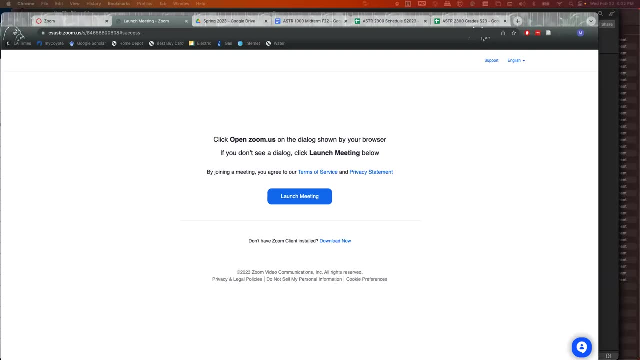 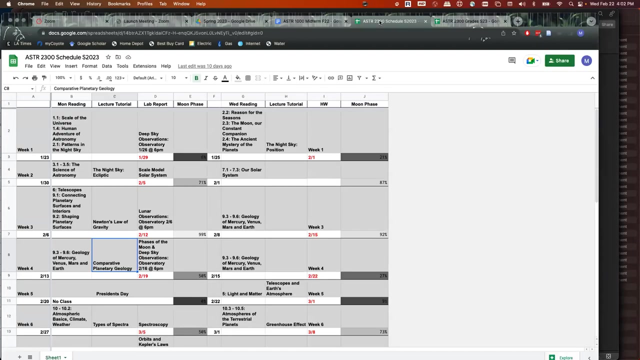 All right. So if you looked at the schedule, you'll notice we're off schedule. That's my fault, Didn't know how to drive good- And so that's cost me $80.. So if you ever need to learn how to do, 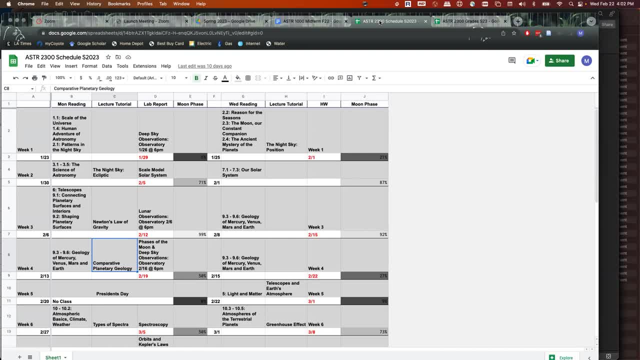 insurance? just ask me, And now I know how to deal with insurance. So what we're going to end up doing is: this is all going to slide a little bit, And it necessarily will always kind of do that, just as we get through the content more slowly. You had a homework. If you can turn that, 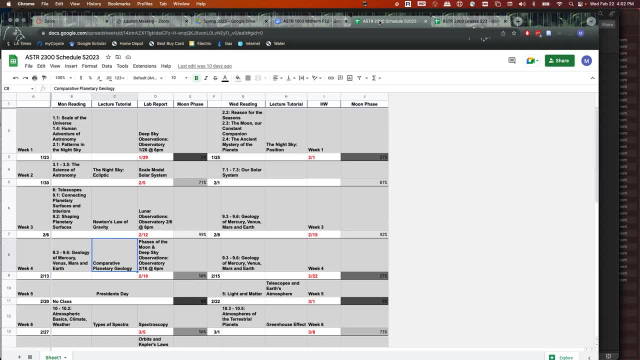 in by the end of today. that'd be great, And then I'll assign. I'll make another homework this weekend, I'll try and grade everything and get everything back to you on Monday, And then next homework will be due the following Monday, The only full week to work on it. Everyone okay with? 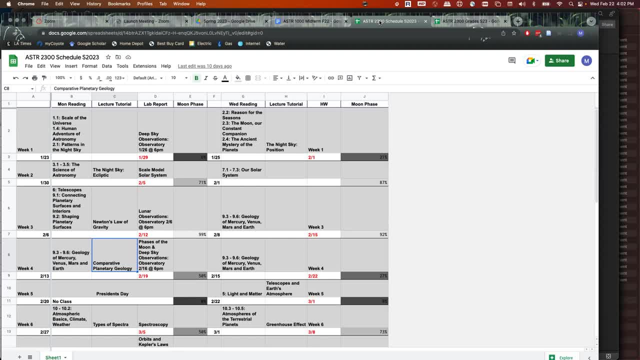 the last homework Questions on it. Okay, Caesar's around, You can always send an email if you have some questions in the study room or for class. to kind of start with, We were going to do a lecture tutorial today, but I don't know how to print and everyone left, So I couldn't print. 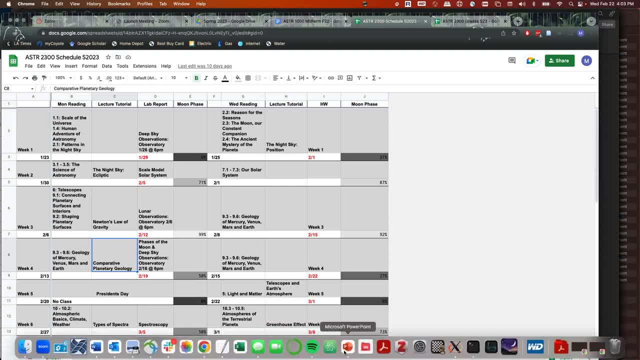 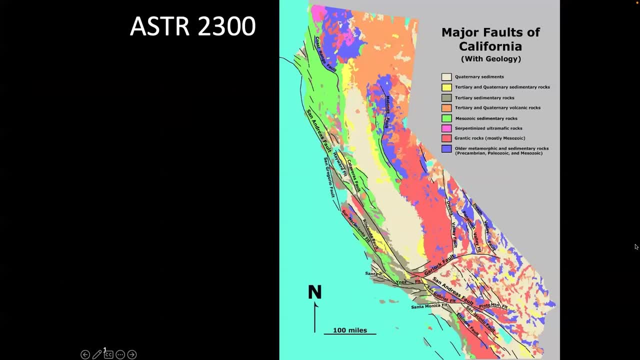 anything. Yeah, I can't print directly from this computer because apparently that's going to cost money. So, c'est la vie, I should have probably learned, Okay. So what's this California? Okay, So I was in Tahoe this weekend. Oh yeah, It was fantastic. I went skiing And it was actually not. 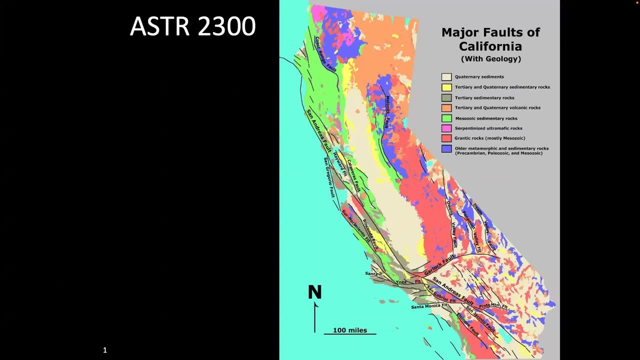 that bad Right as I left, a blizzard started coming. They're going to get four feet over the next week. Come on, Come on. Places in Southern California, in the mountains of Southern California, are going to get between five and seven feet. Yeah, It's a lot of snow. And when we talk about the context of atmosphere, 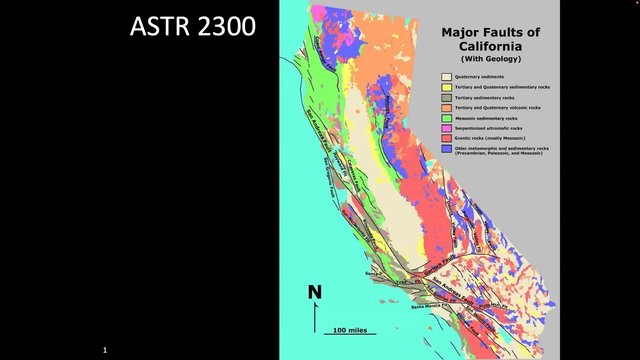 that will begin to make a little bit more sense. But in particular, I was looking around at the mountains because I'm a dork And I was looking at them. I was like what kind of what kind of geology is this? Right, Because we've learned about certain processes. We've learned about 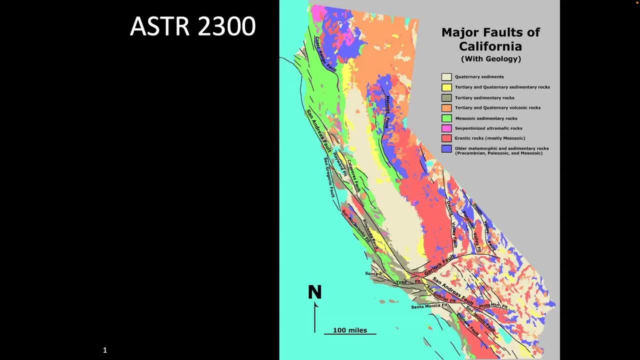 volcanism. We've learned about tectonics, We learned about erosion, We've learned about impact cratering. And I was up here. Where is it Right here, Okay, And I was kind of like, huh, what causes Lake Tahoe to be so high up? Anyone know? Lake Tahoe is right here. 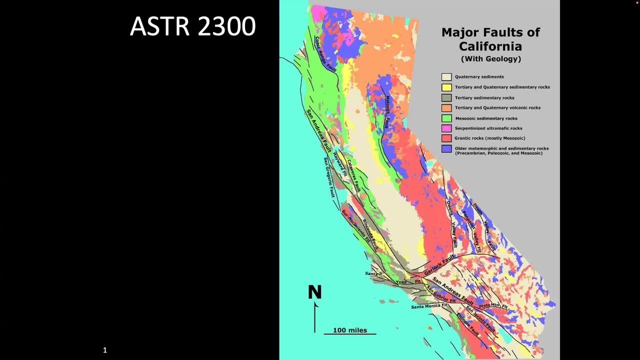 It's not losing that. So this is a map of what. This is a map of what state- California, Okay, Good, Okay, This is the ocean, And the colors here tell you what kind of rock it is. I do not expect you to know what type of rock that is. That's okay. The lines are falling. 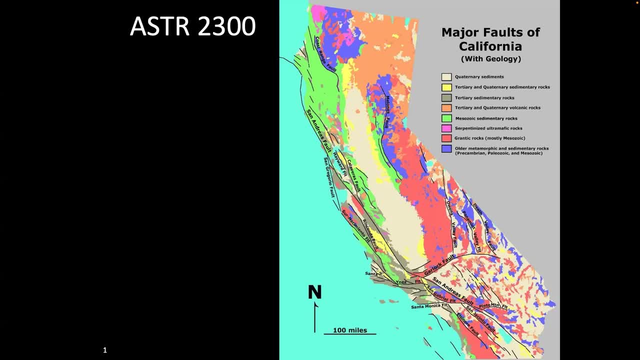 Okay, Yes, So they were volcanic And now they're not. So, in fact, what ended up happening? if you look at these faults, what is this telling you? What story do fault lines tell you? There's a movement, Yeah, Movement of. 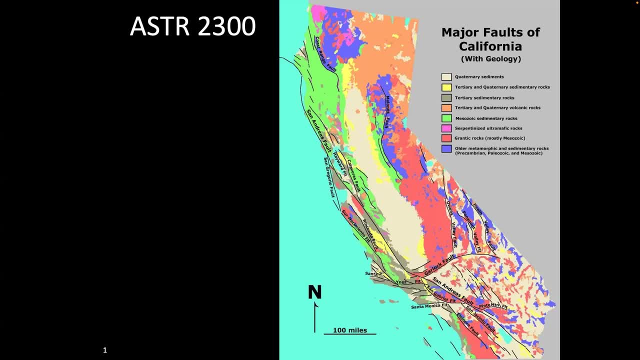 Plate Very good. So we have plate tectonics here And in particular, the fault lines that you see are the movement of several plates. Now, defining something as a plate is not as easy as when you go home tonight and make something on a plate, because that's a discrete object. Here we're really 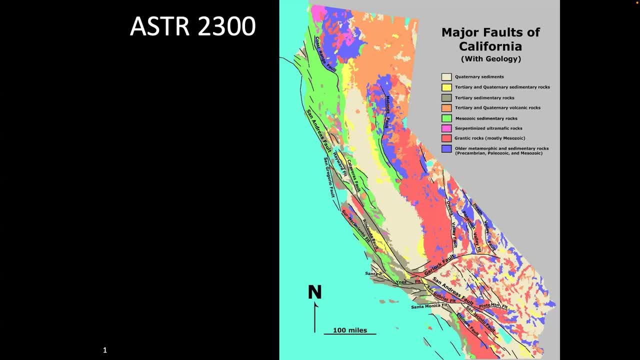 talking about the fact that pieces of the earth are next to one another And some of them move and some of them don't. You'll notice here this is the San Andreas fault. right, That's the famous one, But there's a lot of other ones too, And in fact this one kind of goes perpendicular to it. 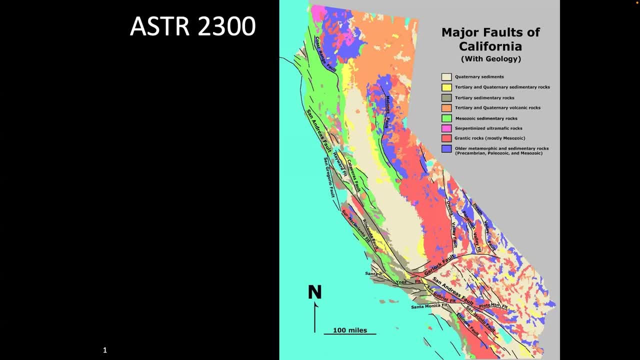 And so you're thinking to yourself: Well, is that a plate? No, But there's different sections of rock that have different abilities to deform. Okay, And in fact we can see the whole history of California right here. Okay, How do I do that? Where is the Sierra Nevadas? Does anyone know what the Sierra Nevadas is? 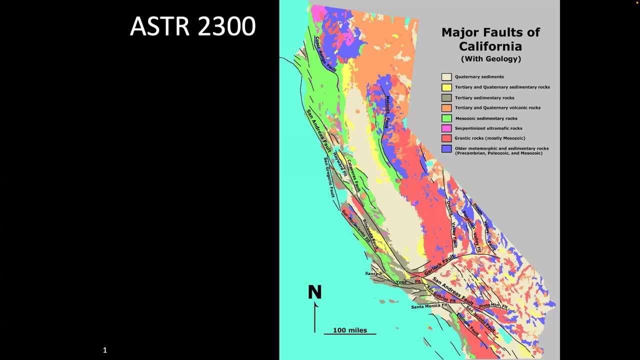 Yeah, It's like a large non-bridge, that's kind of like separating Nevada and California. Exactly that's this, right. and if you look very carefully here, you see that this is mostly granitic rock and you don't know what the word granitic rock is, but essentially this is rock that was melted. 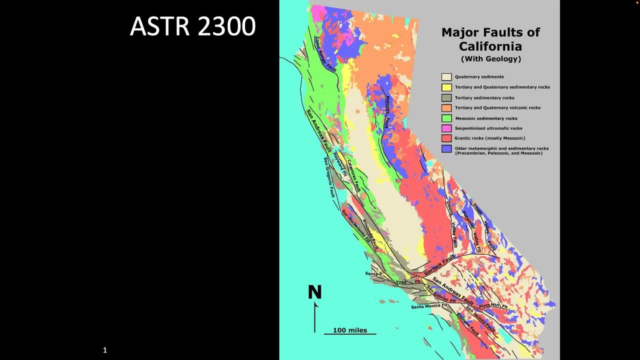 in our mantle and then it came up. you think yourself, how did it do that? so what ended up happening is: many millions of years ago there was a different plate that went under california, melted and then bubbled up. as it melted because it was now lighter, and it floated back up because 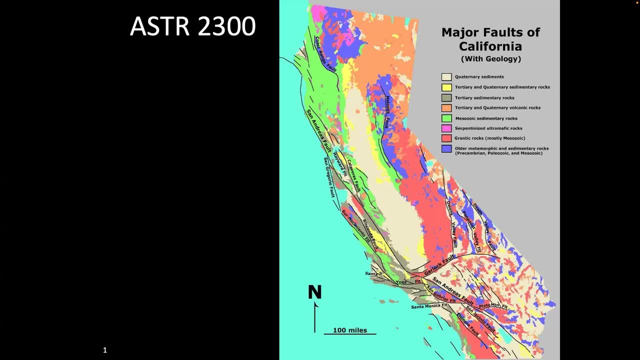 it was hot and it formed a chain of mountains here that were volcanic many millions of years ago. lots of volcanoes just like now. if you go up to seattle, you'll see things like mount hood, which are active volcanoes those are forming for the same reason. mount st helens, the volcano that 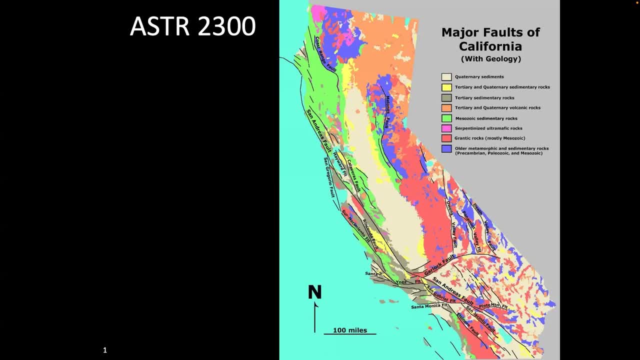 we saw that absolutely exploded. that's a version of the same volcano that we saw that exploded, the same phenomenon, okay, so this plate's going this way and you'll notice it's not straight. that's scary. no, because rock is bendy, right, it's okay, everything's gonna be fine, right? 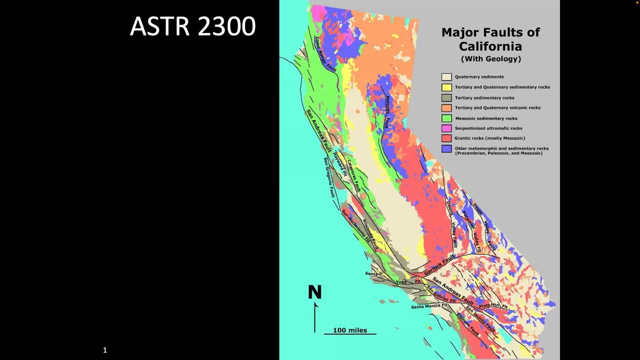 now what happens when this moves? property prices go down. very good, we buy houses when the property values go down, because we've all lived here, it's not scary. but all those people from new york and they finally leave, yeah, then we buy up all the properties. right, do a little paint cover up the cracks in the 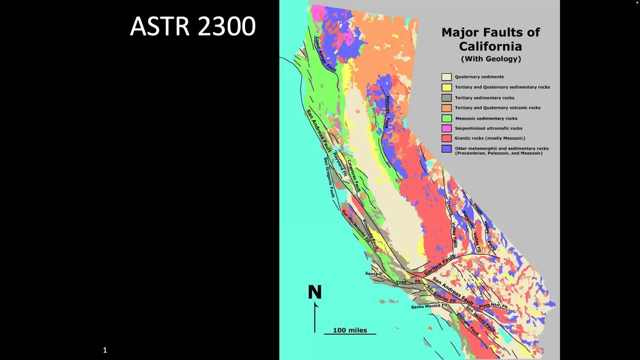 foundation. okay, so we're gonna put all the things that we talked about together today and, um, as i mentioned before, we won't have electric tutorial, but at the start of monday we will have one on what we call comparative planetary geology. just looking through all of 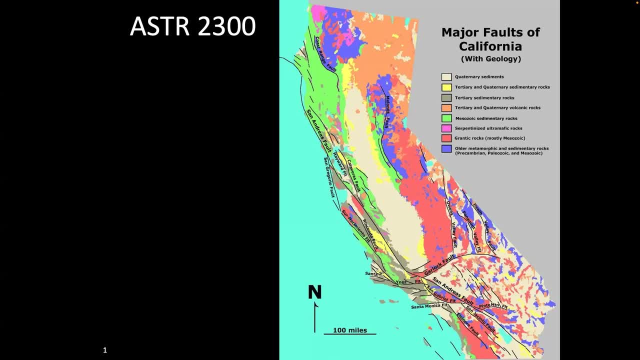 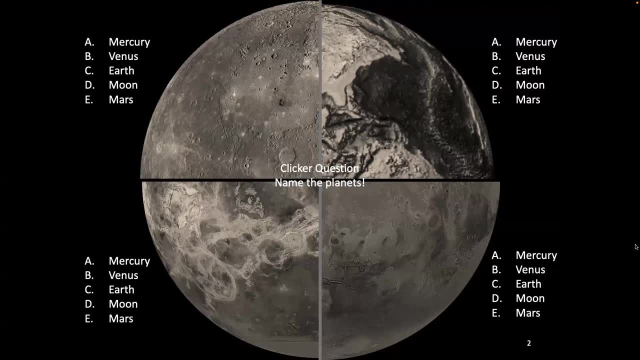 the different types of planets. so we've talked about the processes that we've seen, and today we're going to talk more in detail about why this has all happened. okay, okay, i want you to have a quick look at this and, based on the features that you see personally, 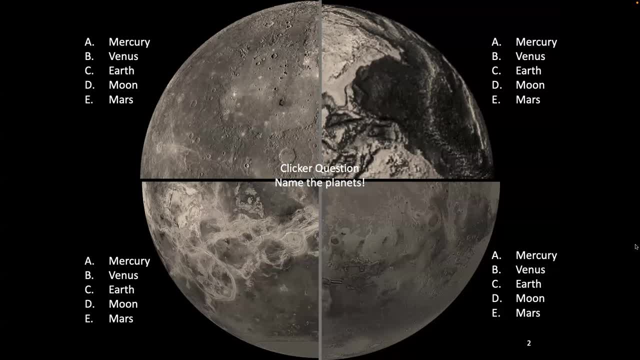 right, um, what is the? uh? why do i have a fifth one? what are they doing that makes them boring? mysterious, different triggers? i think: oh, oh, oh, cool, all right, i figured it out. okay, there's five answers for everyone. okay, is this one in the top right one of these five? is this one in the top? don't answer yet. 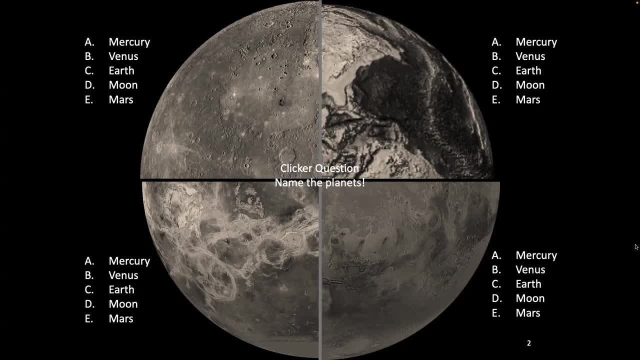 is this one in the top right, one of these guys? okay, well, i have this one. yeah, i did make it kind of harder, okay. so what i want you to do is i want you to write down just for yourself, think about the answer right there, based on the features you see. 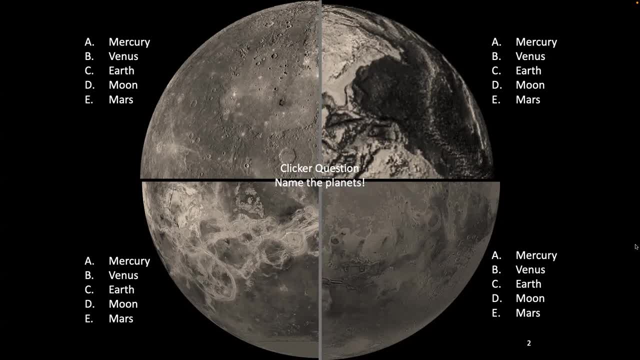 okay. so for this first one, how many people have moon? raise your hand if moon. okay, raise your hand if different answer. what's different answer? uh, i think it's mercury, okay, okay, raise your hand if mercury. okay, so, about half moon, half merger, this one. raise your hand. if earth, raise your hand. a different answer, what's their difference? 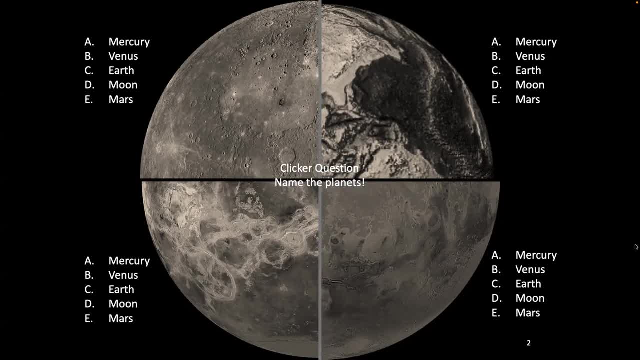 i think this is mercury. raise your hand if mercury mercury's, okay, what's this one? raise your hand of venus. raise your hand. a different answer? all right. what's your different answer if you're going to for me? oh, let's see what this like. marce, raise your hand is marce. 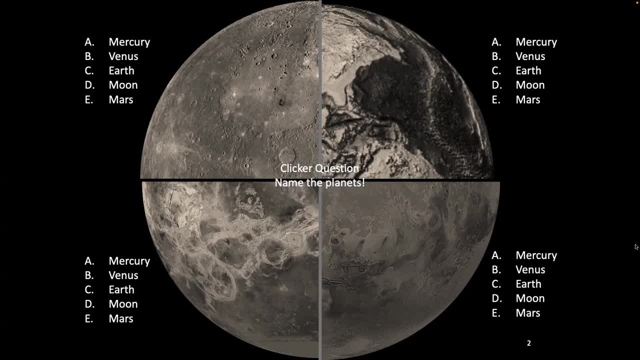 raise your hand a different answer. what's your? i think i think you think mercury. yes, mercury, all right, mercury is the one that no one- no one- really studies mercury too much. some people don't know what it looks like. so in fact, that is mercury. what's that one? what's that? 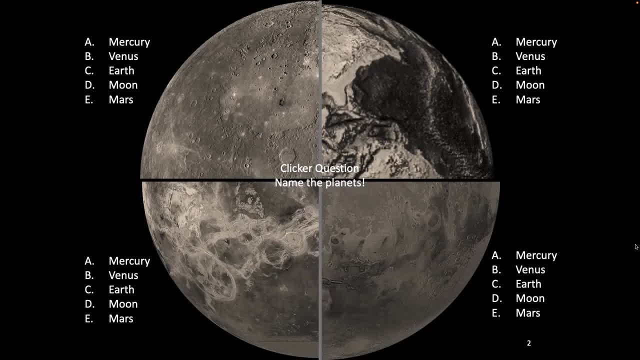 india. that's the earth actually, but this is florida- oh screw it. so the trick that i pulled there that pulledist- oh screw that. so that i pulled there that pulled all the water off and now if you'd like some more so you can clean it up if you need it. that's the reason why i năm mealia'sさん and i'm so jealous: dude. 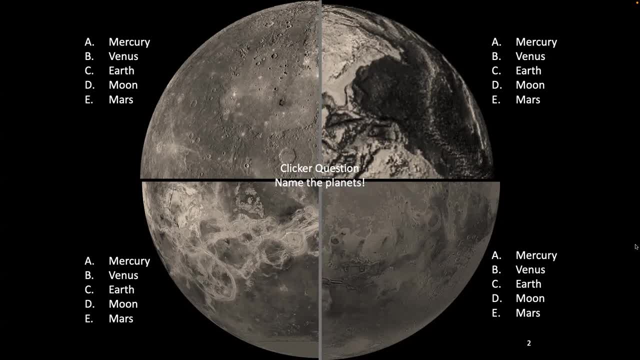 i'm sorry for all the hard work i did but it hurts so much and sorry for your help. if you'd like some more off and i expanded the topography, i can do whatever i want. i'm teaching the class. yeah, it's kind of the earth, but i changed it right. that's the earth. after all, the water gets blown. 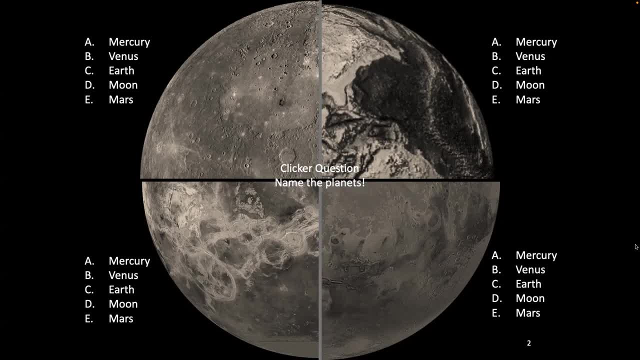 off. wait, is that flat for real? florida sucks, yeah, real flat. it's super flat. it's super flat. if you go to florida and you look around, you can see the whole state. okay, uh, this one was venus. everyone got this one and this one was the one that was going to give you trouble because i didn't put. 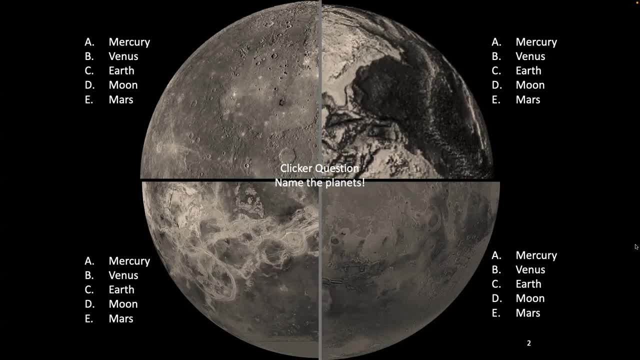 the color on it. that is, in fact, box. so okay, you can tell that this one's mars because of these dendritic features here, when we compare mercury to mars, they're very similar. without color- if i don't give you red, you wouldn't know the difference, except for the fact that it looks. 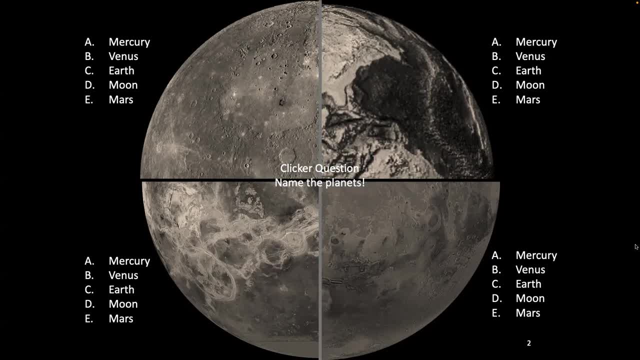 like erosion happens here, and erosion has never happened on mercury. why has erosion never happened on mercury? why has erosion never happened on mercury? why has erosion never happened on mercury? there's no atmosphere. there's no atmosphere. we said. for erosion to be a significant factor, you needed what kind of things? water- water- that was a very good one- or air can work, and 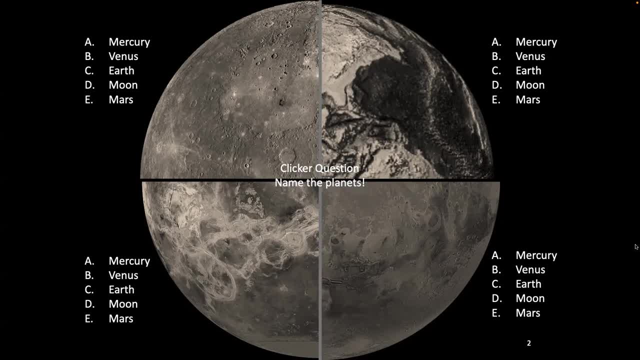 what's another thing that can erode ice? ice is a good form of erosion. in fact, it's what carved um the yosemite valley. glaciers move, yeah, the water is so. for example, you can have co2 ice, co2 glaciers which carve rock. okay, but you're absolutely right. 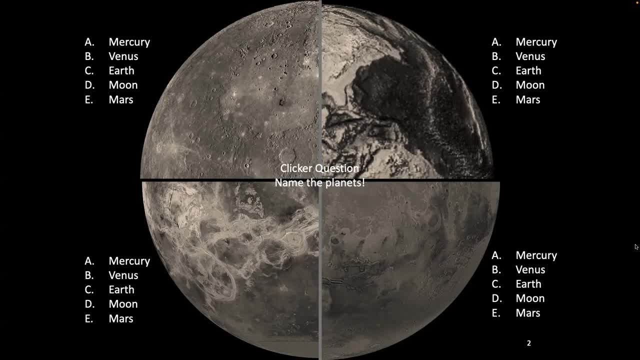 so fluid, i should say, and if you're in my fluids class, water is a fluid, but also there's other forms of fluid like, for example, liquid nitrogen. now you don't think about that as critically important here, but maybe when we move out to the outer solar system we'll see some funny stuff. okay, this one was obvious. i think everyone got. 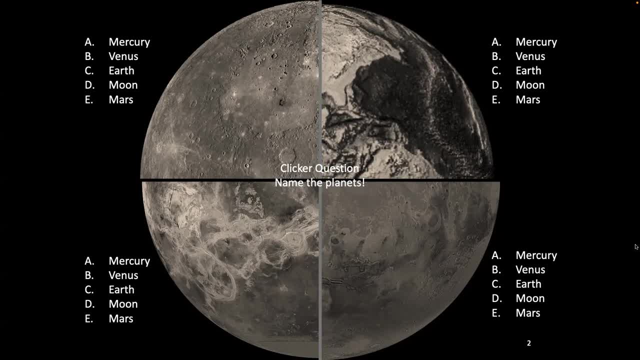 this one? why is this one so obvious? that's a lot of scarring- scarring, yeah. what about craters? i want a crater right. that's kind of it kind of like shows that it's venus or earth right. and then, once you see this, you say, well, i don't see any countries that i recognize. 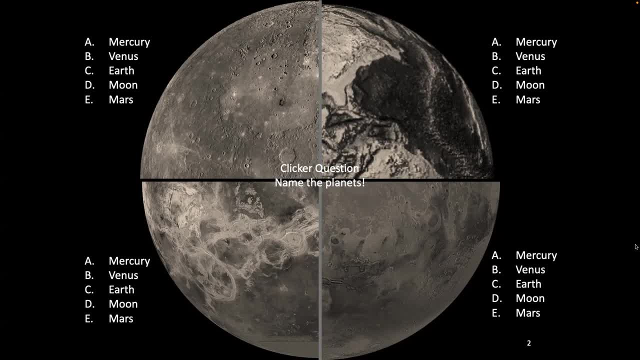 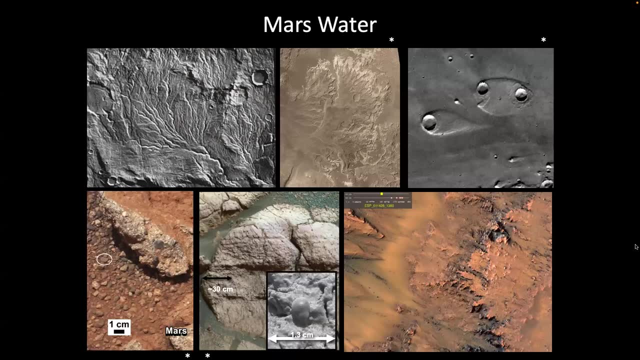 not okay. okay, so we talked a little bit about erosion. let's finish the discussion. i know it's been 15 years since you took this class last, but mars in fact has water. those when, when i showed this in the bottom right hand side, i said there's erosional features. 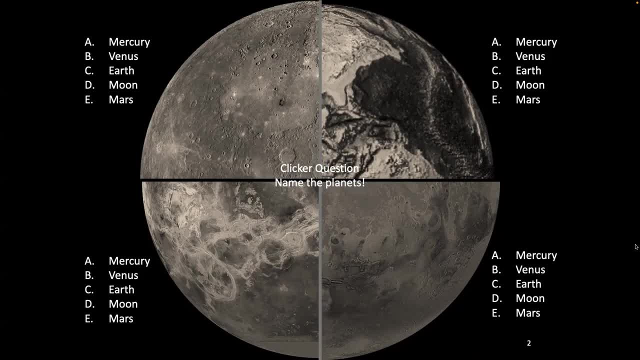 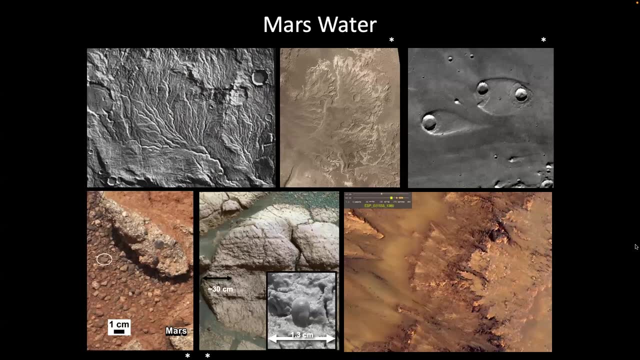 okay, i didn't actually show you last time that there were erosional features on mars, but here they are. so you hear probably every year that they found water on mars. um, that's not wrong, but it's also not helpful. as a you know, it's like a way to like sell magazines. 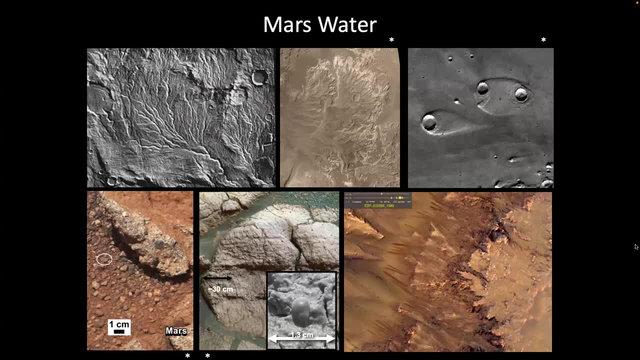 and stuff like that. so we're going to talk about that a little bit more, but let's get started. so the thing we're interested in is to find different forms of water. so we've known for a long time that there's water, ice on mars, there's water vapor in the atmosphere, and sometimes we 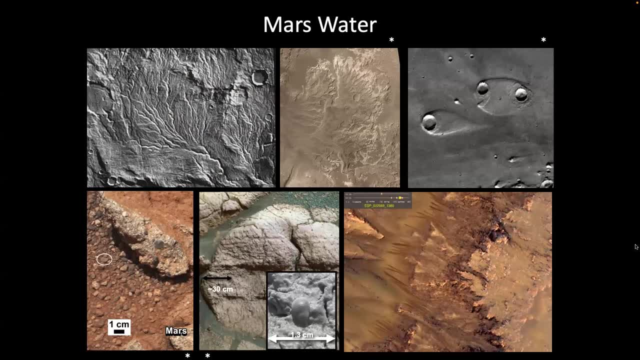 find different forms of water, ice, and that tells us about the history of water on mars. so in the top left hand corner, you see, uh, what we call dendritic channels. these are channels that form when material is flowing into a larger river right. so this looks like, uh, modern southwest america, right desertification. 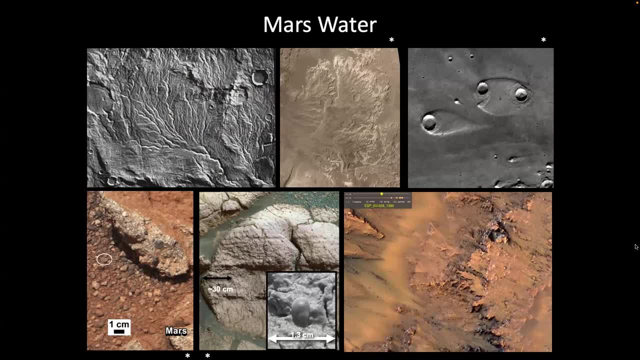 and then this one here is a form of an estuary or something that is like coming from a river and then depositing material here. what we can do with very cool cameras. we can look at what the composition is and we see that all of this material in the fan with what's called. 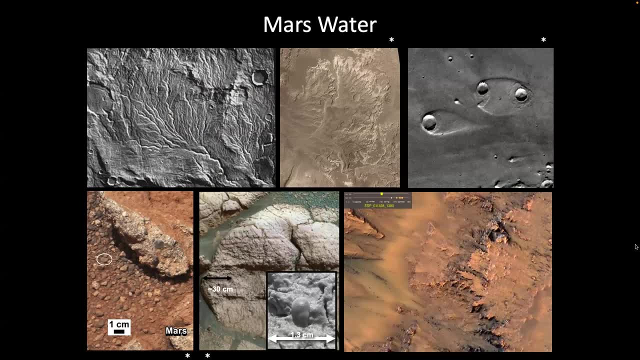 an alluvial fan is of the same type, so this river was bringing material with it, and then you have a slight change in the elevation and it deposits that material on the ground. then the water disappears and you're left with the rocks that it brought with it. 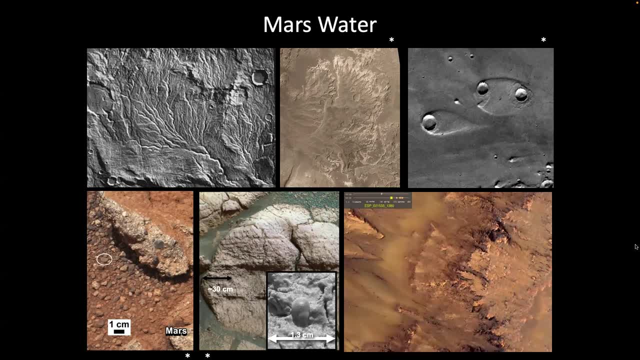 this one's kind of funny though. what's this? okay here. volcano, anything else, volcano in a crater? where do you see the volcano? where do you see the crater circle like this one? yeah, what's that? bubbles, okay, i hear bubbles. yeah, there's a crater and a bunch of wind. crater and a bunch of wind, okay, okay. so remember that. if 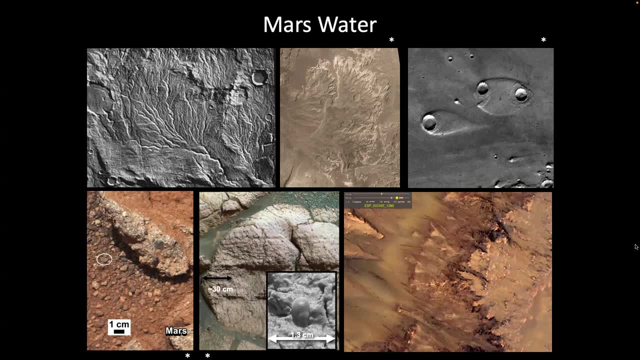 these are craters, they must be relatively big, right? so this is like a large structure. okay, don't know how many kilometers, but probably maybe hundreds of meters a kilometer, something like that. and then you have this shape, and that shape reminds you of, sure, some form of erosion. in fact, if you put a rock here into a stream, you would see water go around. 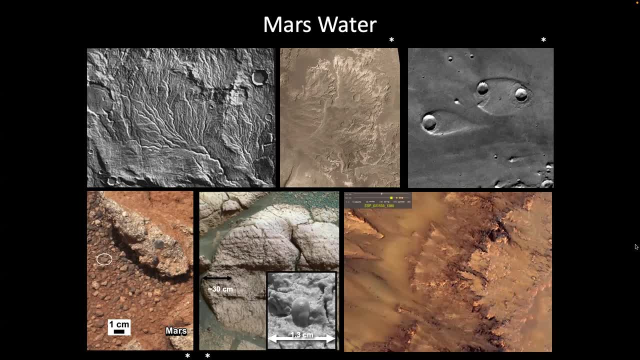 it like that, and that's what's happening here. this was a stream or something moving to the right hand side. there was an impact that punched a hole in it and formed walls, and then that material went behind it. the same thing is true of these. isn't that weird? 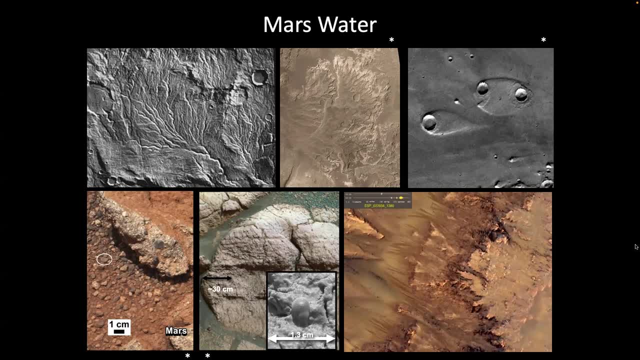 okay. so what's this shape and that shape reminds you of? so we see that there is like water on the surface, certainly flowing. all of this is evidence of water flowing out of mars. you can see other stuff. there's these fun things called blueberries. this is what happens when rocks tumble. they like smooth out. you see the river rocks. 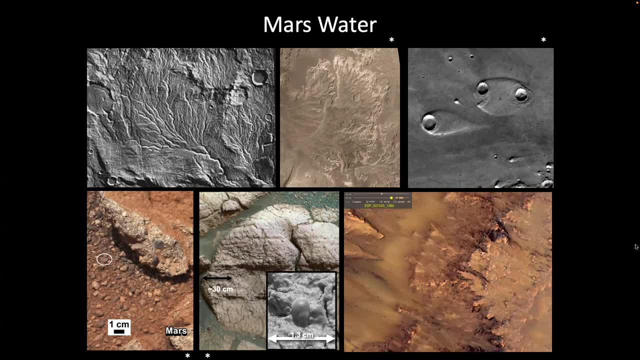 and in the bottom right hand corner is what happens when you have really high resolution imagery. so this is a cliff and you're seeing icy sort of saline water on the surface of moths. this is the biggest one in the past like 10 years, because what you're seeing is basically called a brining solution. anyone ever, uh, cook their? 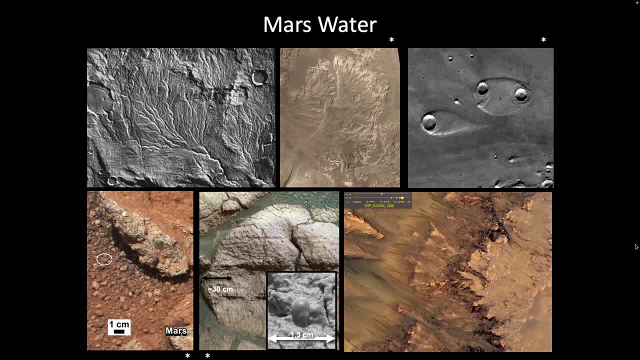 turkey in brine. it's brine. brine is salt water, so it helps to really retain moisture in the bird. um, and the same thing is happening here. you can make the mixture of water very, very briny, very salty. then you can uh, change the freezing point enough so that it sort of flows. that's what. 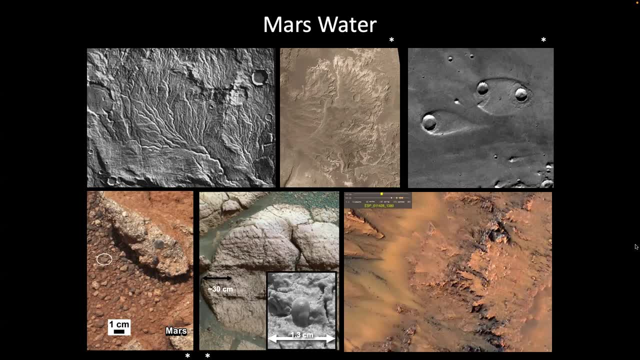 happens here. it's trapped in the edge of this cave wall and then, as it's exposed to light, it moves along, moves out of the edge of the cave wall, goes down like water does, and drains out, cool right. and so people want to know: well, okay, bugs, any bugs? that's our question. that's why we 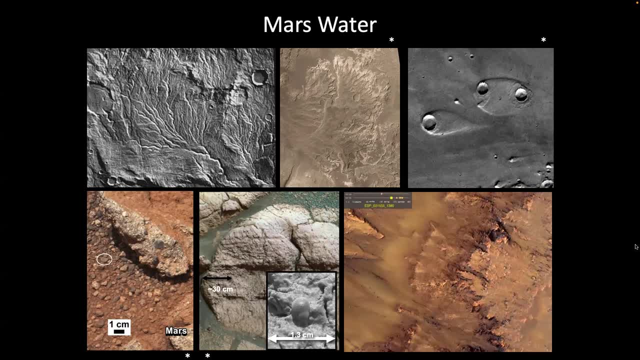 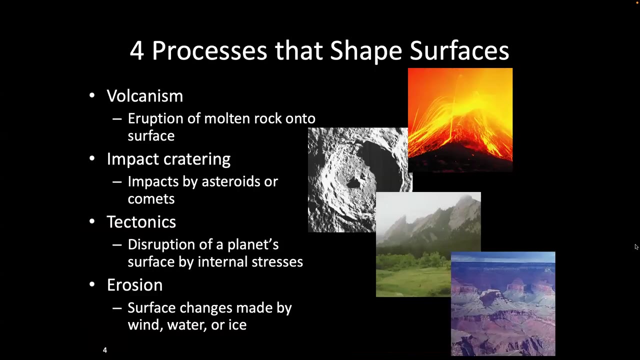 like mars looks like it has ancient water- probably did for a long enough time. did life ever arise on mars? is the nobel prize winning question right? are you gonna win it? i'm not smart, let's go all right. so here's the four processes. these are the ones i'm going to come back to time. 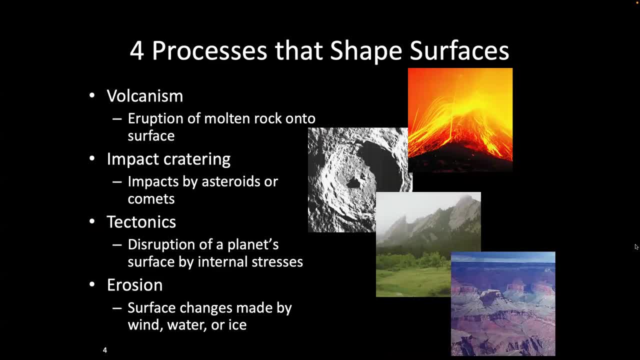 and time again. okay, first process: volcanism- eruption of molten rock onto the surface. there's different types of volcanism. what are the three types of volcanism? slimy volcanism gave you goopy at goopy volcanism- this is talking about the viscosity- and it gave you different types of forms that you saw. 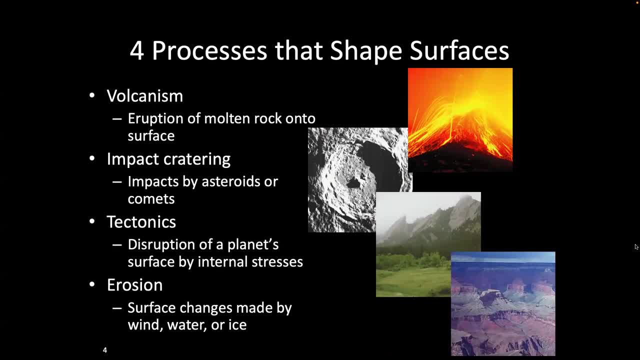 steel volcanoes is one of them. ronnie volcano gave you like a flat plane, right like maria on the moon, distant nite earth that you can go visit. weight loss, Doppler ge, insignificant number. there's two fun things that are: earth can rub, compute four twentysốf euchovian heights. and what's a good example of that? not that, how squirming, hahaha, the one they go bang violently, go the straddle. good impact rating. what's that? meteors, yeah, stuff hitting the surface, performing the surface. good example. on the moon? yeah, that's clearly what on the moon? what's an example here on earth that you can go visit? 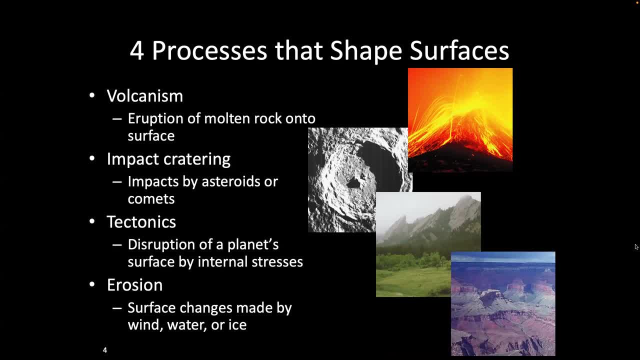 Yep, which is called Easiest thing: Crater, Almost Meteor crater, Great naming, Okay, tectonics, Yeah, but what does it mean? Good, so very important. right To notice that she didn't say place. 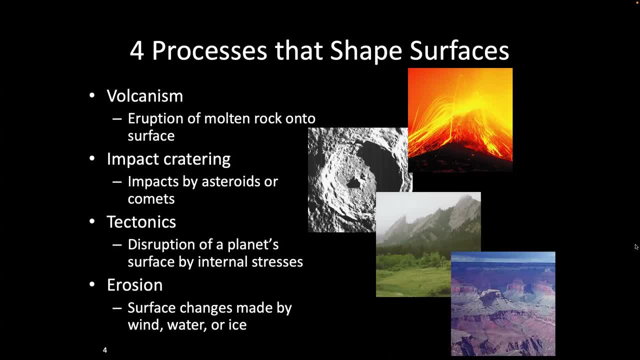 It's a movement of the surface. That's the correct thing to think about, Because on places like Venus there isn't necessarily plates that go under one another. It just could be like squishing and moving apart right On Mars. we don't think there were plates, or at least we don't have evidence for that yet. 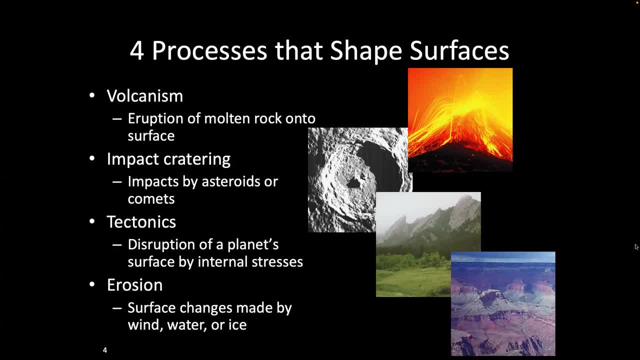 Sometimes it gets uplifted. So here, if you decide to go to Colorado, you can see Boulder, And Boulder has sandstone from the ancient sedimentary floor of an ocean And as you walk along the mountains here, you're walking backwards in time. 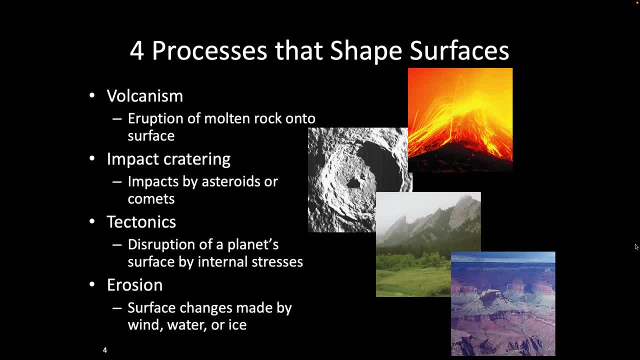 It's pretty cool: You can see different fossils from different millions of years. Okay. finally, erosion: We just talked about that. I'm not going to go over that, Unless you want to see it, Okay. Okay, Let's talk about a planet. 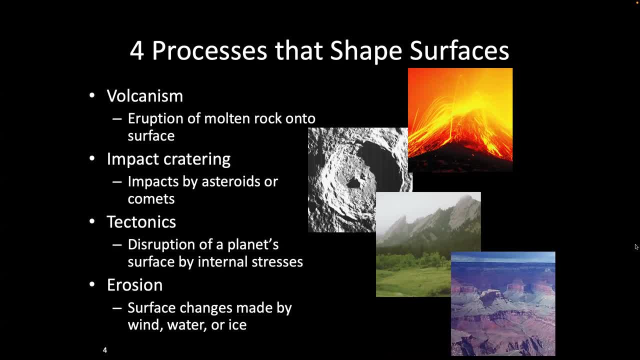 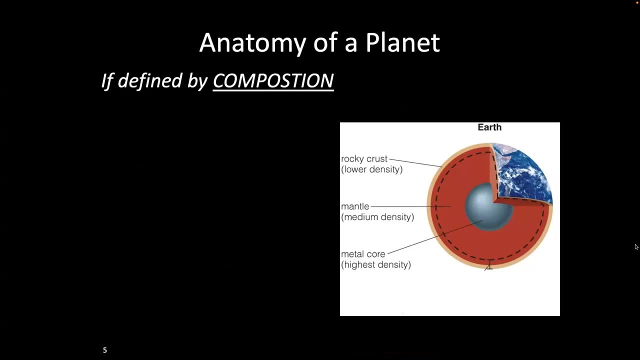 What are the parts of the planet when we think about composition, Or Just the planet itself? we'll get to atmosphere later. Yes, that'll be later. Mantle, What's that, Mantle, Mantle, good, Alright, and then the. 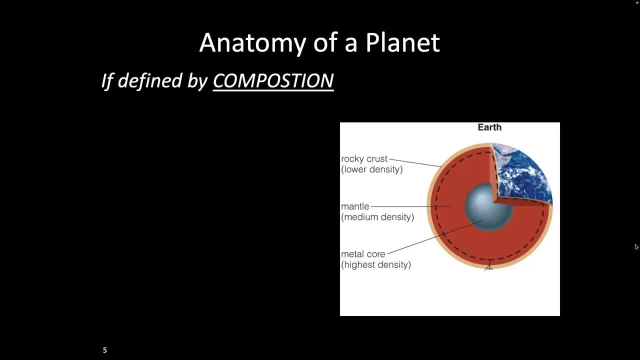 Crust. So here we have the core, the mantle and the rocky crust And they have different densities. Why do they have different densities? Yes, but why is the highest density stuff in the middle Heavy sinks? We're going to go back to a lot of really simple rules in this class. 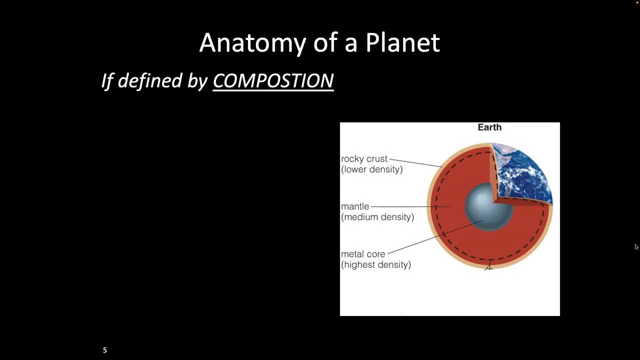 like hot rises and heavy sinks. Okay, So in fact, this is hottest in the core. Why would that be Exactly right? So you have all this mass on top of you. It's crushing it. So it's hottest in the middle, but it's also heaviest in the middle. 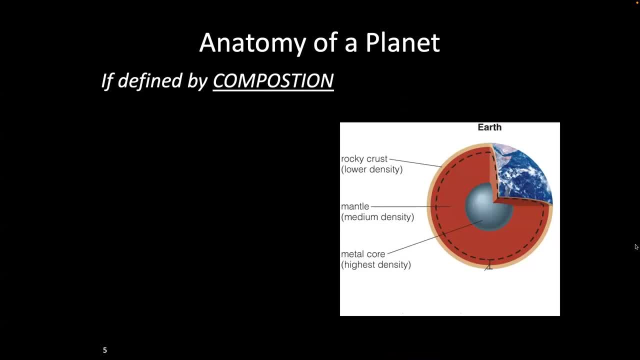 Okay, Where is it the coolest Where we live? Very convenient: You go underneath the surface too far. you melt. We don't like melting. I like the current temperature, Even if it could be a little warmer outside, right Okay. 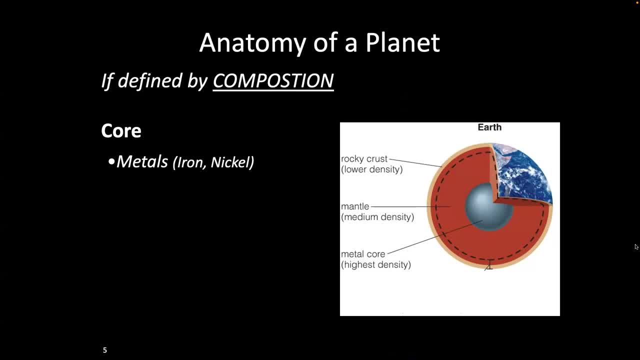 The core is made of metal, Mostly iron and metal. Okay, The mantle is made of what we call silicate rocks. Why are they called silicate? Because there's silicon in them. Yeah, So silicon is an element that's formed inside a supernova. 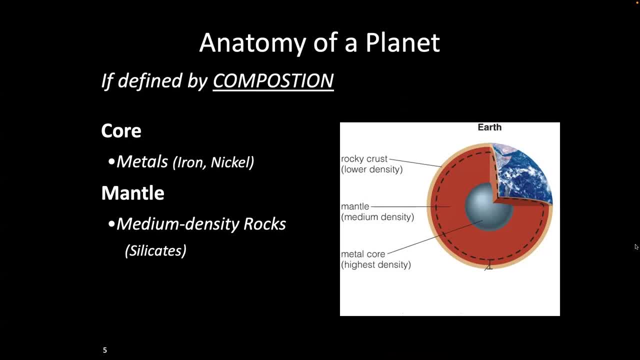 It's put into what we make our planets in And it's less, It's dense, so it sits outside. So, for example, if you take, let's say, you make a salad dressing tonight and you put oil and you put vinegar and you put a little water in there, dilute it in some peanut butter, you shake it up, 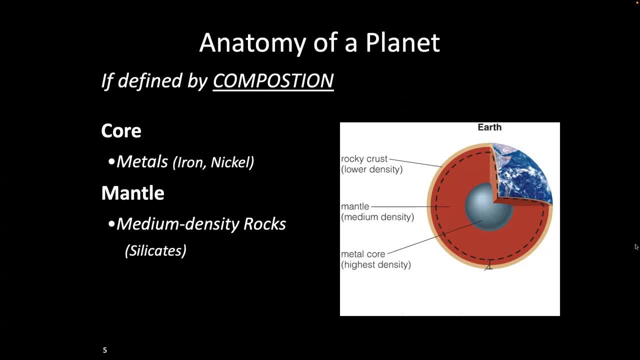 I don't know if you're making it just keep moving for a second And then you sit it down and you forget about it and you go play video games for seven hours and you come back and they're all separated. I don't know. 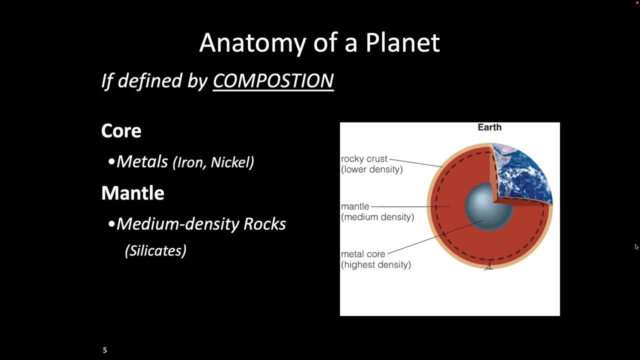 Whatever, Which one is on the top, Water, Well, okay, The lightest one, The lightest one, The one on the top, and which one is on the bottom? The heavens right. And the same thing is happening here. 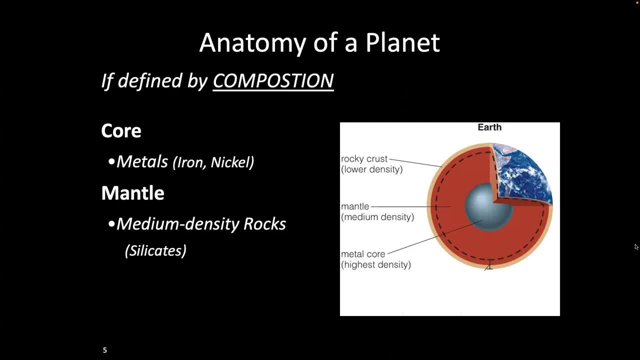 Okay, So this is a process called differentiation: Heavy stuff sinks, lightest stuff floats. So what do you think? the crust is made of The lightest stuff? Very good, Okay, So that's what we show. In fact, these low density rocks, like granite and the salt, are the ones on the top. 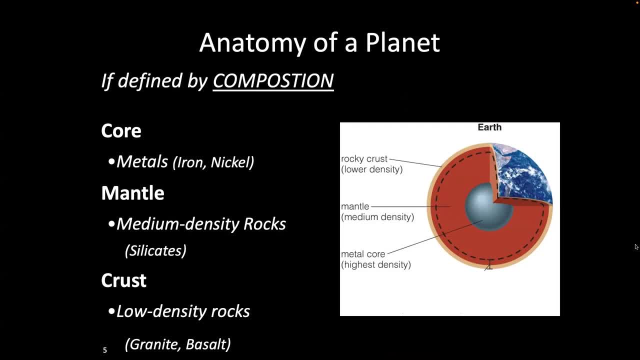 The composition here between the mantle And the crust. the actual stuff that it's made out of is very similar, but the way that it's made is very different. So granite is really great for rock climbing. Why is it really great for rock climbing? 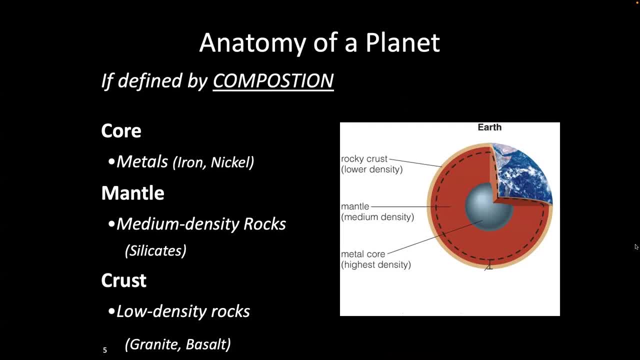 It holds its shape well. It's very sturdy. Okay, So I put my hand on it. It's not going to explode, But what's a great example of a type of rock that will explode when you put pressure on it? Sandstone. 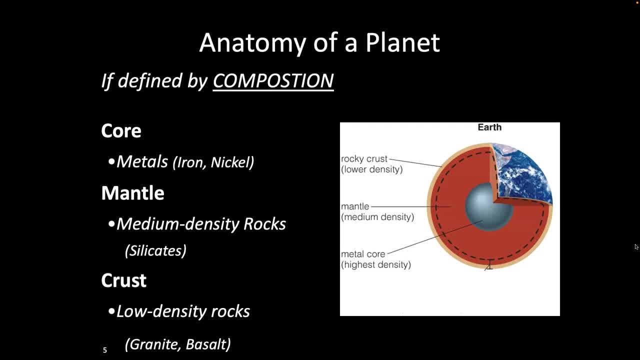 Yeah, That's what we call choss. So you put your hand on it. It's really like it's formed by putting layers of old, dead skeletons together of bugs. You put your hand on it, It's gone Okay, Whereas the stuff that's granite is formed in the core or, sorry, in the mantle here. 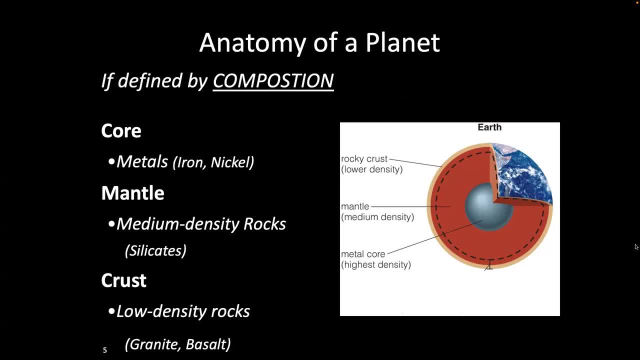 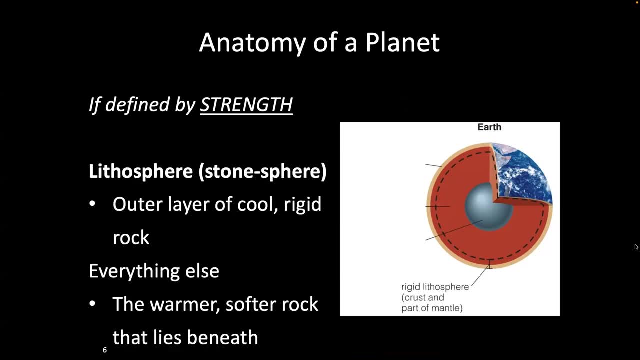 And then it moves back up as it gets warm. Okay, Okay, So that was composition. Let's talk about strength. at the very top You have this Fun word called lithosphere. Oops, this was supposed to show the show words, but how to say them? 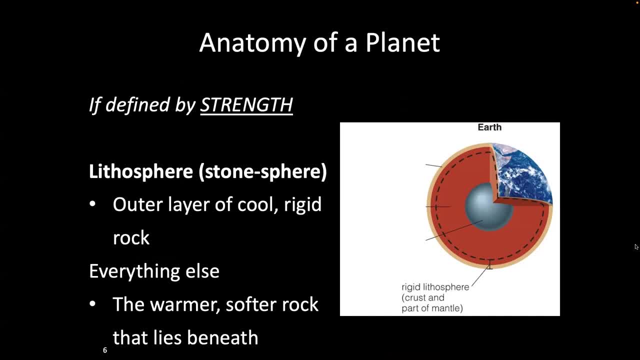 Um, lithosphere. when we talk about atmosphere, uh, lithosphere is the place where we live. It's the stones here, the exterior of our planet. So everything else below it is, um, just everything else. Man is looking for it. 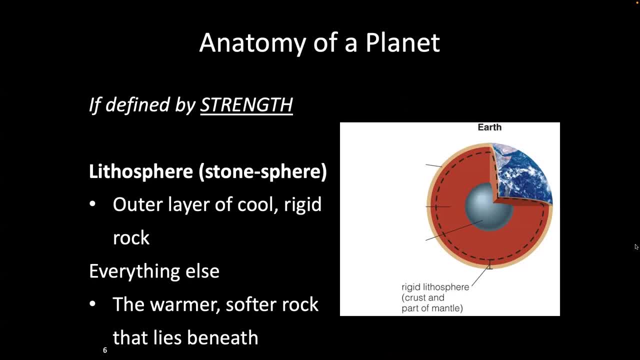 I can see it right outside. I'm totally blanking. It'll come when, when we do this again on Monday. um, I'll remember what are the words are underneath there? Um, how do we know that this is inside of our planet? 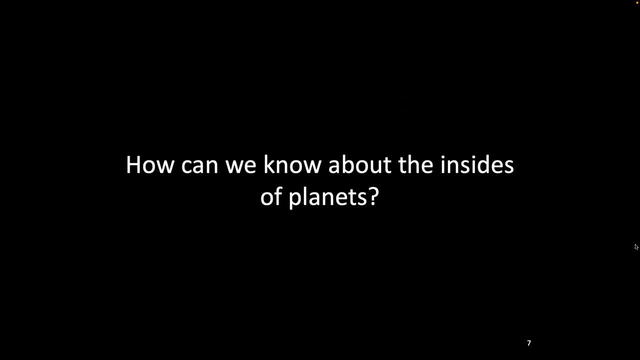 That's the magnet of fixed force out of the body. Yeah, so that gives us composition Absolutely. How do we know there's a core Magnetic field? Definitely We know there's a magnetic field that defies the core. Yeah, 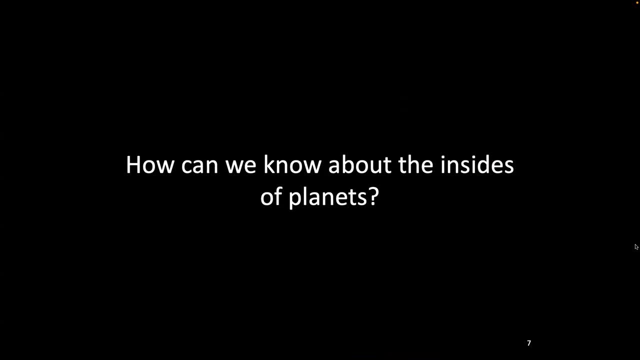 How do we know the shape sign? Does anyone bend to the middle? So, despite the fact that, like all of you would say, oh, the core stops spinning or we can drill down to the center of the earth, that is not possible. The deepest we've been is like a very small fraction of the surface. We've never gotten down into magmatic chambers in detail. Why? Because lava's hot. We die right. So in fact we know about the interior of planets because of 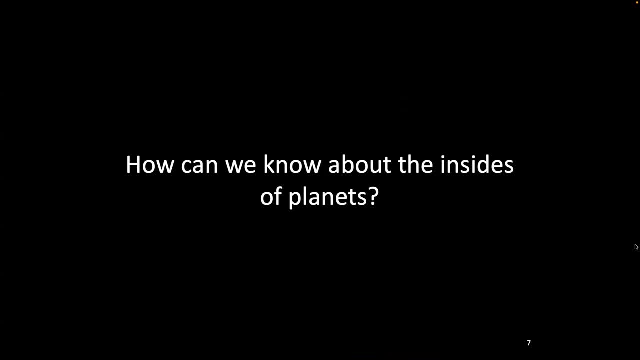 We're going to do this in two ways and I'll tell you really quick in a second. Let's use our brains for a second. What if we just wanted to do composition and I didn't have very much information? Let's say we're thinking about a different planet and I give you the mass of the planet and how big it is. 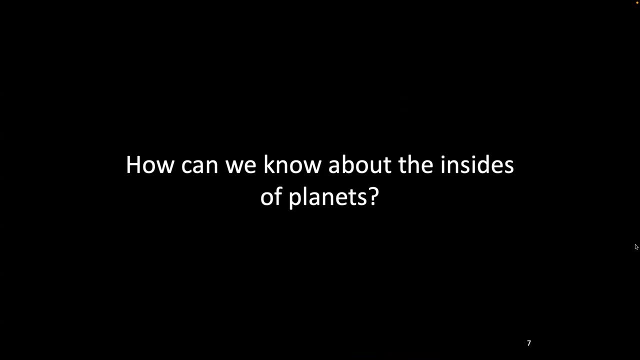 What could you kind of tell me? The density, The density, right, If I add those two things together I get density. And what can I compare that to? To give us a broad sense of what it might be, you know, 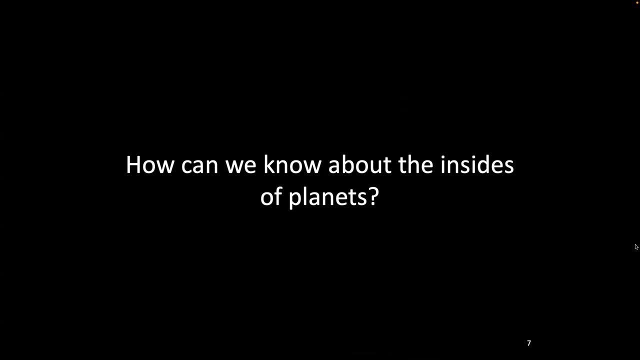 Okay, a little bit more than periodic table. What would you use in particular? What are some examples of things that you would know that planets could be made of? Yeah, compared to ours. what should it be made of Rock? Okay, so the word rock has a density. 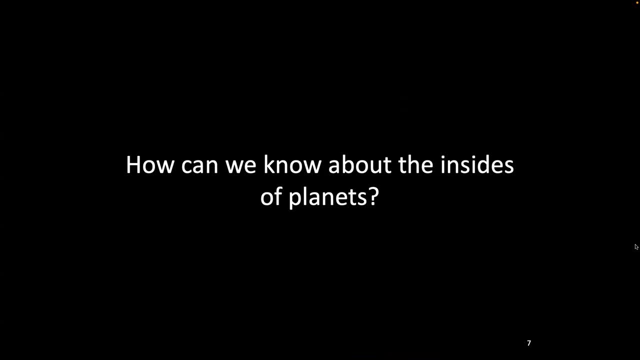 What are other things that are dense that we could compare to Water? Okay, good, So water is the one I wanted you to get to. What's the density of water? One word, One word, What Good. So that's the one we want to have in the back of our mind, okay. 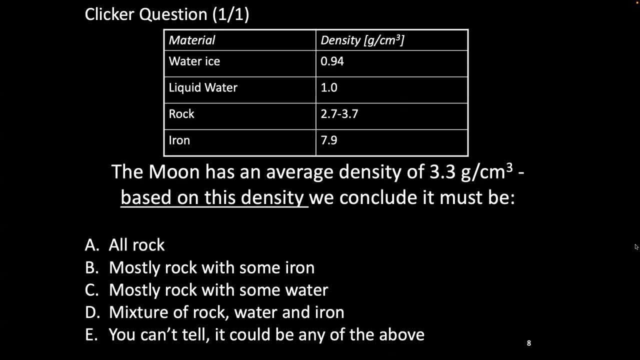 So if we look at water- ice- it's less dense than water. Did anyone know that? That's why it floats. So remember that ice is less dense than water, so it floats on top of water. so if you ever need an analogy for what we are doing here, the top of this rock- okay, it's ice. 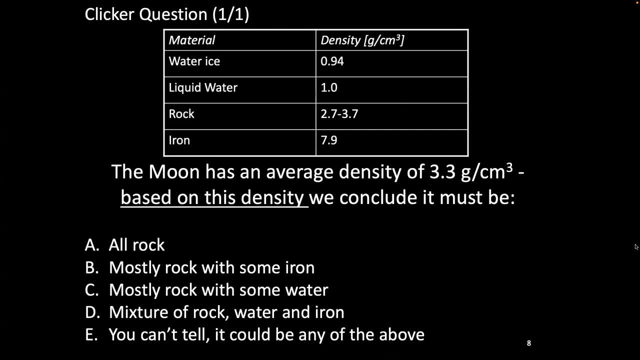 on top of water. okay, ice is cooler. frozen form is less dense than the melted stuff underneath, okay, so just imagine next time you're drinking your water. oh, that's me on the top, okay, all right. rock is approximately 2.7 to 3.7. i'm even going to change that. let's say that it's. 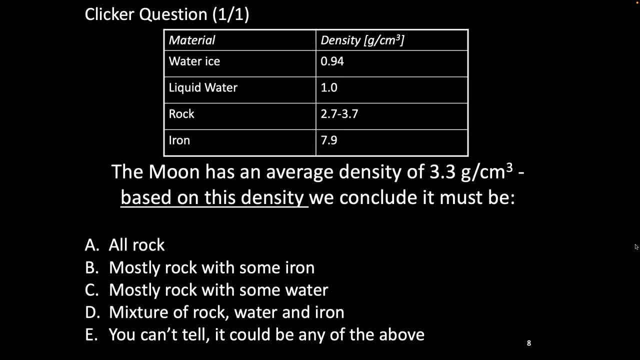 like 3.5, and iron is heavy, very dense. that's why we use it to make important things- and it's about 7.9 grams per cubic centimeter. so let's think about the moon for a second. okay, the moon has an average density of 3.3 grams per cubic centimeters. based on this density, we 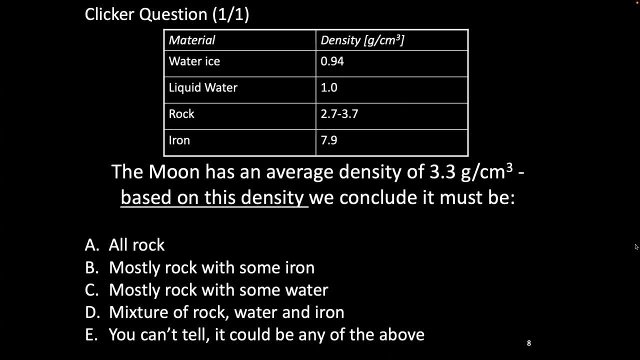 conclude that it must be: a- all rock. b- some rock, mostly rock with some iron. c- mostly rock with some water, a mixture of rock, water and iron or e. you can't tell, it could be anything. i'm looking at this second. let me know when you're ready to vote. 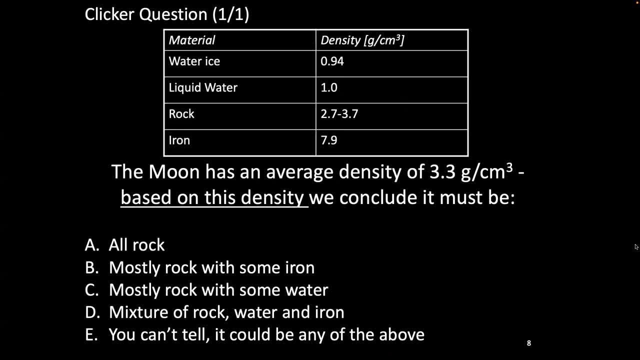 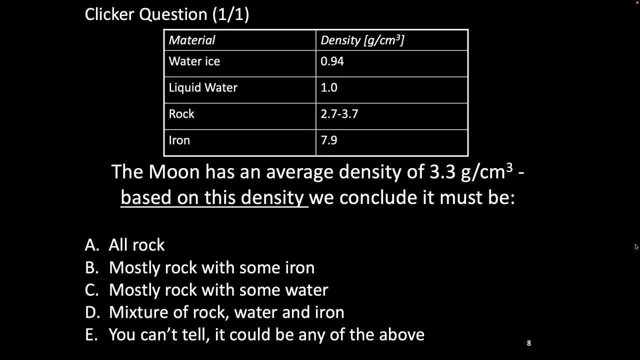 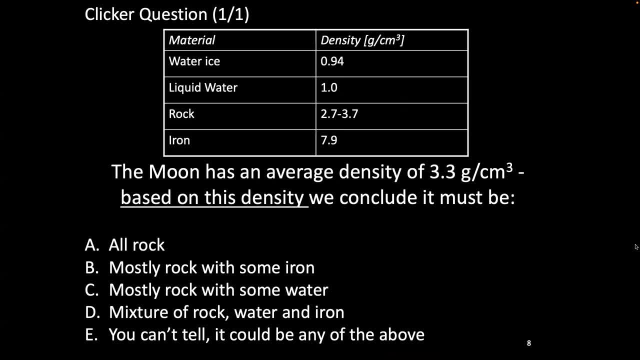 okay, we ready to revote, is okay. or, um, on three, three, two, two, one, three. okay, i only have ones and twos. all right, who wants to make an argument for their choice? yeah, iboard think the one that just is just going off of this kind of 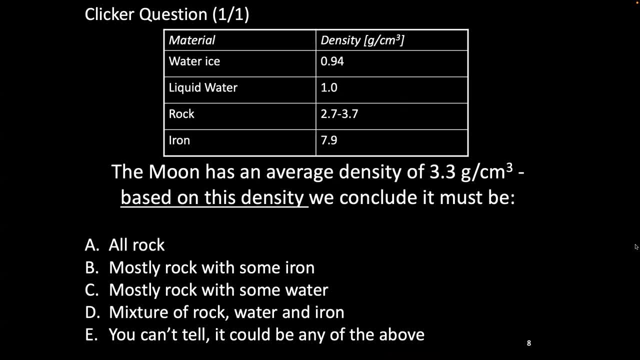 it's right in the middle between do what's that? and their concern. So it's just there. can't be anything faster. That's what he out of. density is the majority, Okay, Does everyone agree with that? And we have a different idea. 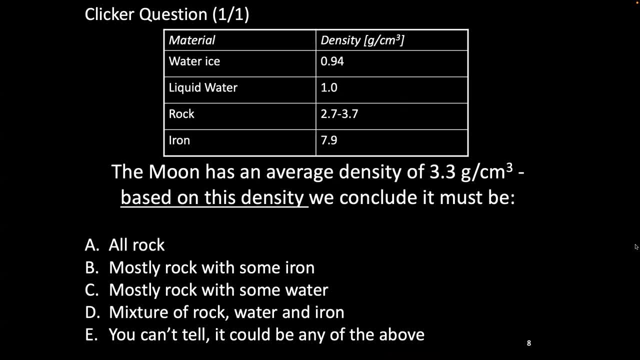 Yeah, I thought too. I thought you based off like outburst, super dense in the middle, That's more dense. Oh, maybe it's connected. Some of my better show now, Dr Been, I don't want to change your answer. 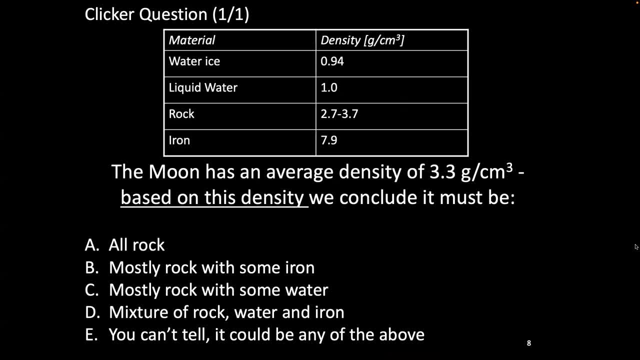 They have a different thought about that. now I would still have a question. So yeah, that's the average. How do I perform an average? Yeah, How would I do the average density in a black? Yeah, The weighted average, right. 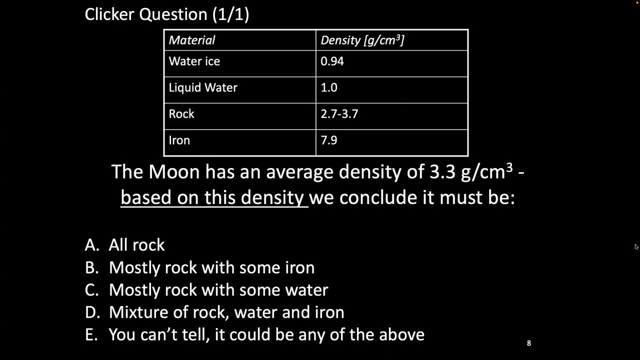 Oh, I don't know. That's too smart. I don't want to do that. If the moon was created from a chunk of the Earth, is that being informed the same way into? No, we don't know any. This is we're doing simple. 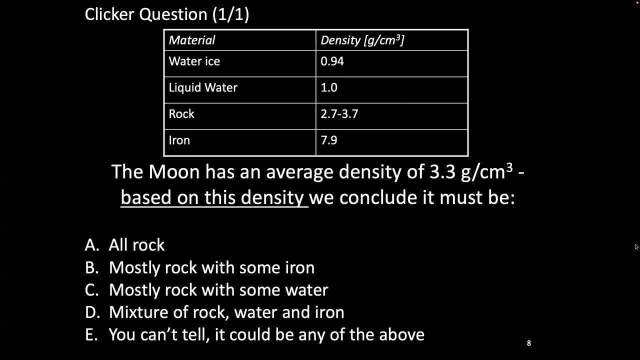 Okay, very simple, simple book, And I just want to say something like: how would I form the average things when I do like your average things? Good, Good, Okay. so you find out how tall the person is and you divide by their. 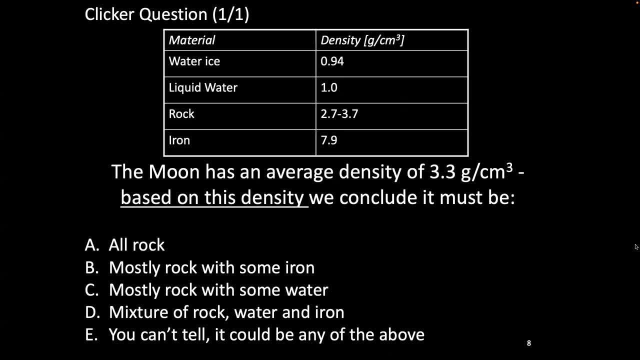 math, assuming they're cylinder, That's science, right. So we would say, okay, we have a sphere and we have the mass and the volume and the heat of Irish, and that gives you an average density. Okay, That enough. No, why not? 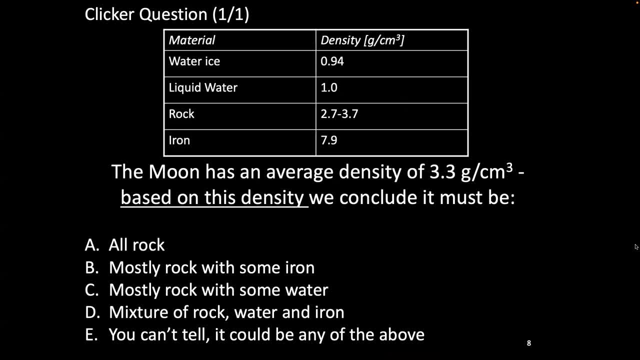 What? No, you think it's good, Everyone agrees. What about this thing? What about this thing, The globe? So it's, you know, like maybe a pound, Very big, Like a foot or something across, two feet across. 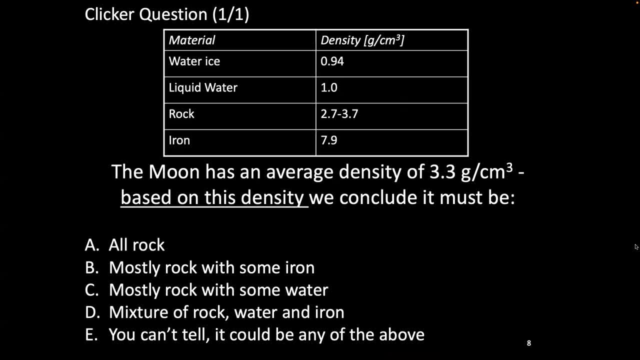 I don't have no idea Right. So I could divide those two and let's say I get something like the density of water. They do it. No, what happened? One number is one number, Good, And it doesn't tell me about the distribution of Max. 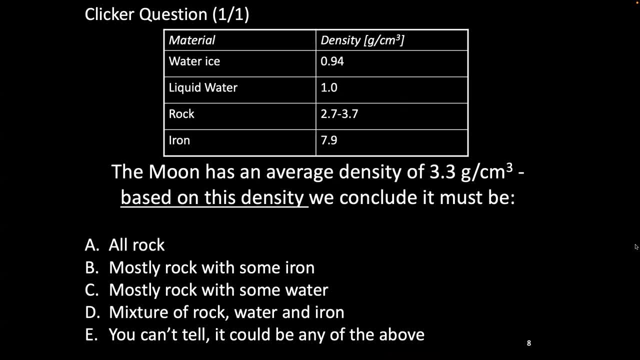 So there's different ways to get to that average density. In fact, here I have an object that is hard identity, and then inside here Not so much right. The air in here is basically zero, So we can't simply use this one or this one. 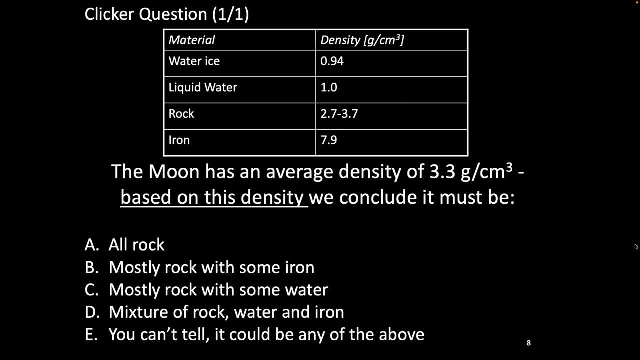 So I got to keep you on your toes. I can't always be as a non-answer. In fact, you can't tell only by the fact that it can't be all of them, but it very certainly could be a mixture of rock, water and iron. 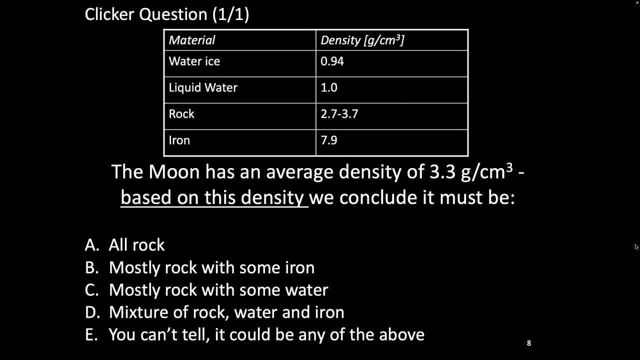 Because, for example, take the average of iron and water ice, Add this number to this number. eight plus One, nine divided by two, four point five, four point five, That's pretty close to three and a half. So now, if I just add more water than iron, 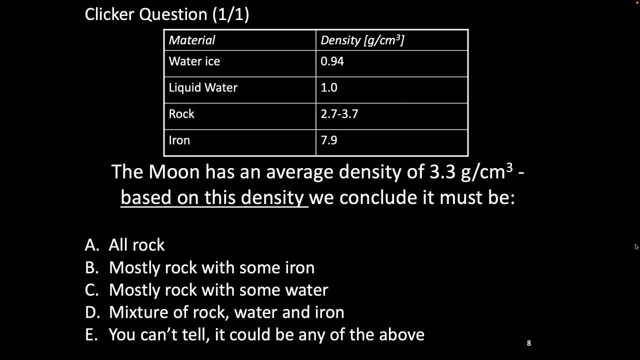 That's going to balance Right. So there's tricky ways to make the composition Correct. What if I said instead that the average density was one? You think it was all water for most people Very little bit Like yeah, if I only have these things to build with, it would be really hard. 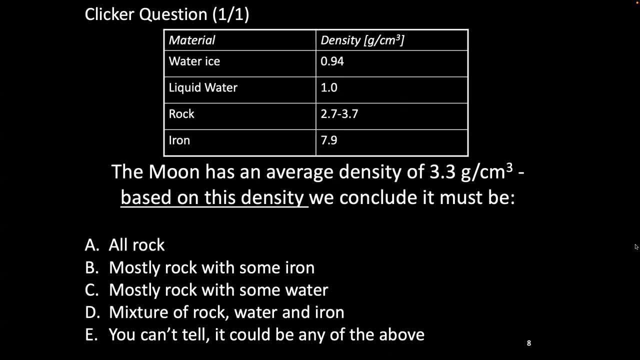 There might be a tiny tiny bit of iron or tiny tiny bit of rock. It is really hard, Right? What if the average density was 18? You didn't do fit, Okay, Iron's not even on there, Right? 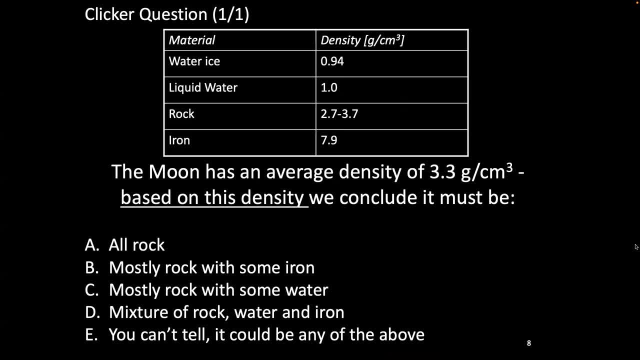 Okay, In fact it's not going to be that. I don't even look at what. would you guess that the average density of Saturn is? It's less than water, Weird. All right, We'll get to that later. So how the hell do you tell the inside? 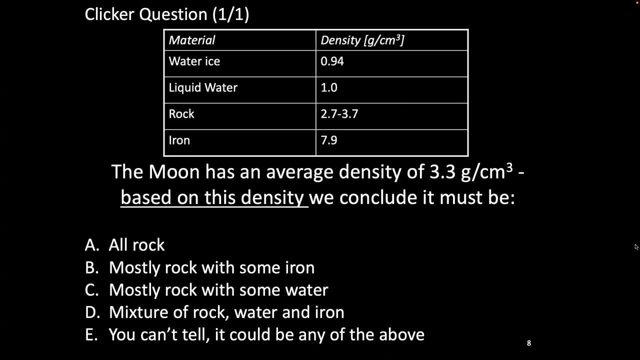 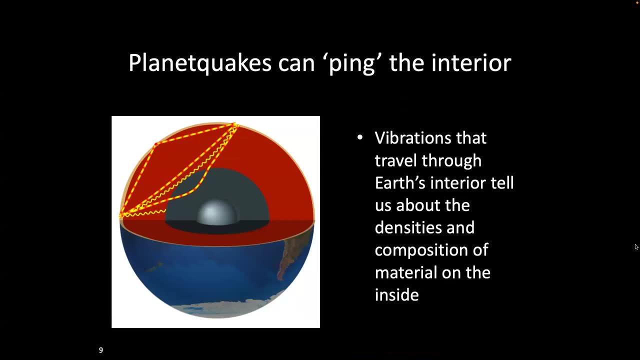 That was this really stupid example of a tail. I didn't learn anything. I already said it. I said it before we started talking about. So this tool that we just talked about is helpful to give us a first approximation of what we're looking at. 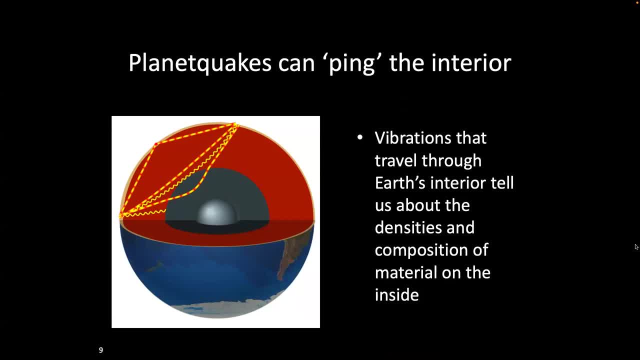 And in fact it tells the interior in a lot of detail. You have to do very detailed measurements, but we don't really know a lot about the core of Venus, Because it's quite hard to learn about Venus and we can't tell what the core looks like. 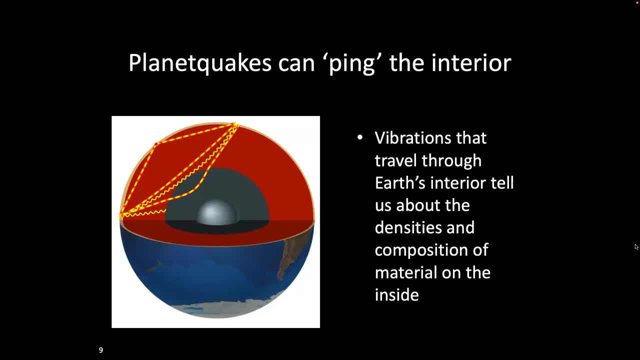 We can tell what the Earth looks like because we live here and we put seismometers down. I put one right here. I put one right here, We'll put one in the back of the room and then something happens in the interior And we watch it at different locations and it tells us about the distribution of mass inside of the planet. 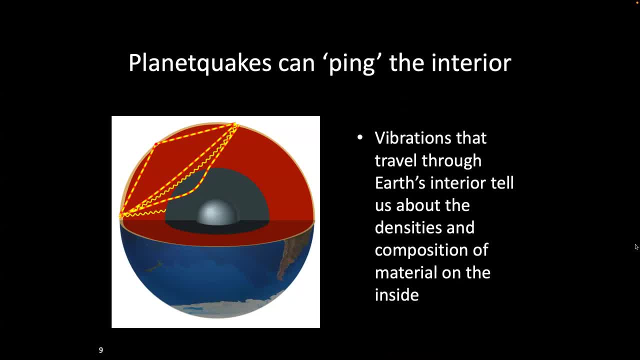 So, for example, there's an earthquake over here and there's a detector on the surface here and here, The way that it propagates right through the Earth will tell us What it's made of. So if they can Signal at the same time, 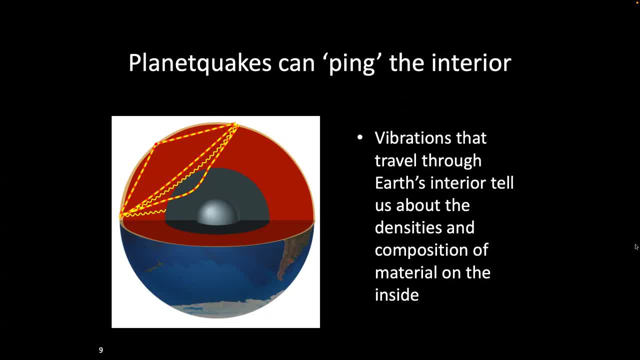 That'd be very weird. The shorter length, So this one gets first. This one gets in. There's a bounce, Sometimes there's a bending through certain parts and there's absorption. This is an entire field of science, All So. 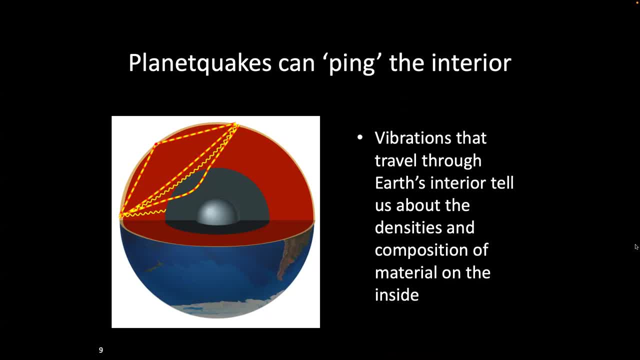 I apologize. Yeah, we landed on Mars and we put a seismometer down and we saw Mars, Quick Waves, Oh Yeah, no, that's okay. I do it all the time, But I also say Earth when I'm like talking about it, did not not earthquake waves. 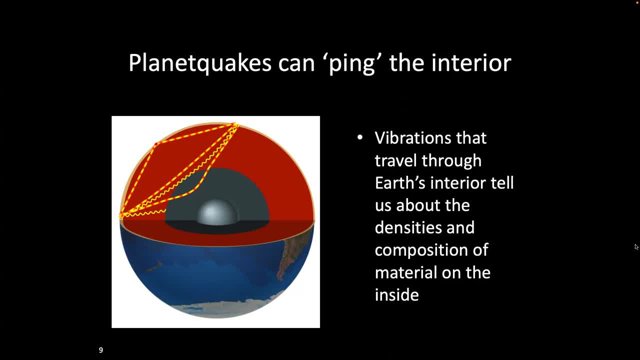 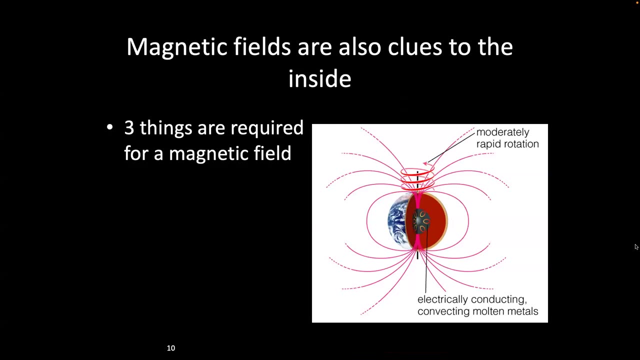 Okay, And so, interestingly enough, this is very well study And it tells us about the mass distribution for very high level of detail. Someone also mentioned that there were magnetic fields, and this is correct, So the interior of the plant can be deduced that there is a molten core by the fact that there is 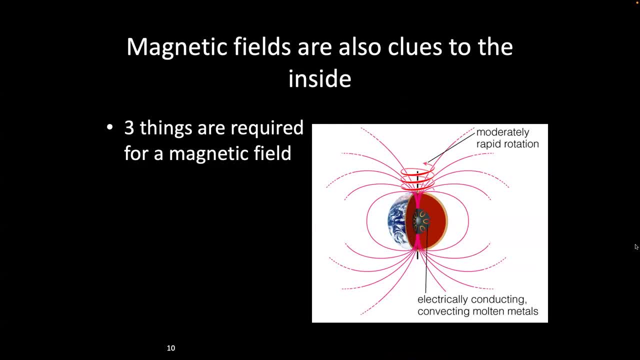 A magnetic field. The reason for this is- and I don't know if you've taken PNM, But there's three things that you need for magnetic field. You need it to be electrically conductive, You need to be convecting. 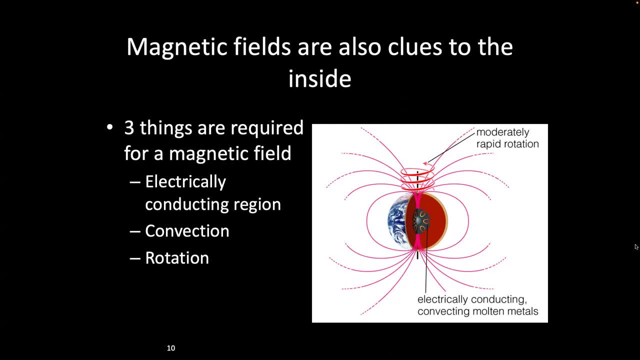 And you need to rotate. Okay, electrically conductive just means that there's. it has an ability to bring charge. So either free electrons or free ions. In some cases, this electrically electrically conductive fluid does not have to be plasma or magma. 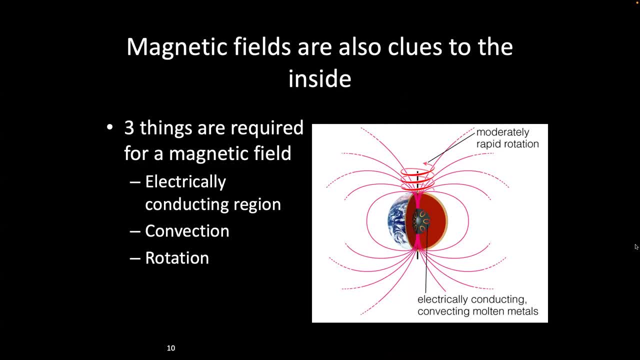 What else is an electrically conductive fluid That might be a lens inside of them- Water. So, in fact, there are places in the solar system that might have water under their crust, And you're going to know that you're a robot and Europa has salts inside of its water and the salt inside of that water is electrically conductive. 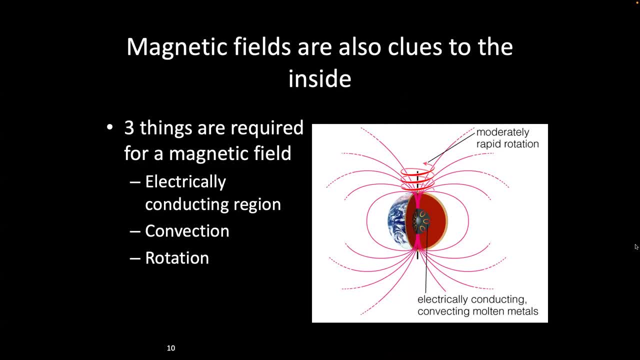 So as we pass by it, we can tell that there's water underneath it. that's responding to the magnetic field. Now it doesn't have its own internal magnetic field and that is because that fluid is not convective. We haven't talked about convection in detail. 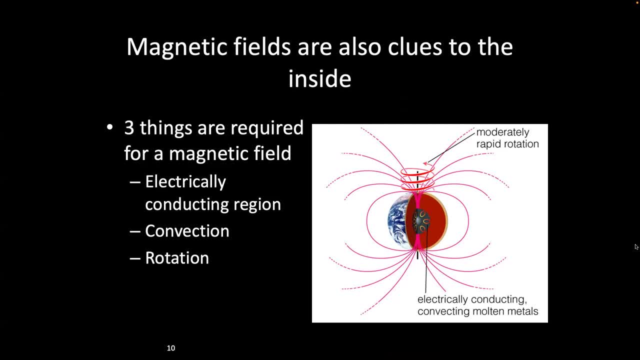 But what is it? Someone who's maybe like seen convection before Oven, So I turn on convection. What does that mean then? Air goes in circles, Hot goes up, Cold goes down. Hot goes up, Cold goes down. 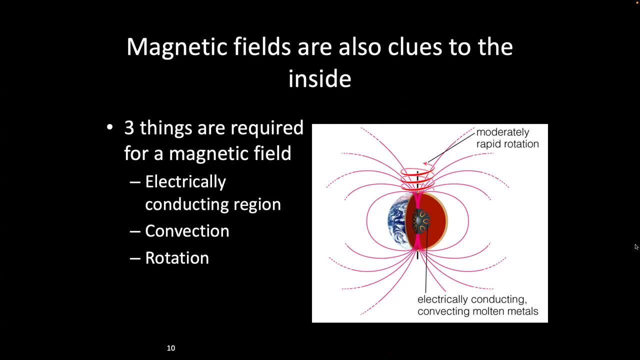 We'll talk about this in more detail. And then rotation, For reasons that are complicated but fun, You need one fluid to pass by another one to form a magnetic field. So you have all three of these. You know that there's a metal core that's rotating differently than the exterior. 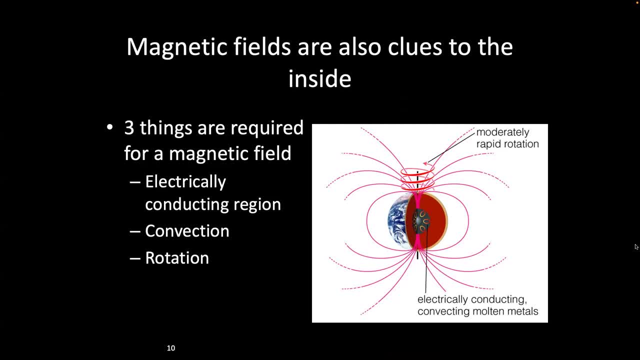 Okay, And the word modestly rapid is ambiguous on purpose, Because when you say rapid, like compared to what? So for some people rapid means like Earth-like, One rotation every 24 hours. For some geochemists they say no, that's silly. 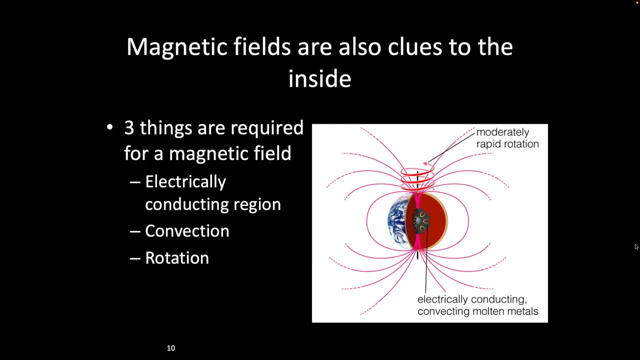 Venus could be considered rapid in the celestial sense. Push it one every three hours, Three hundred and sixty days is one thing. It doesn't feel rapid to us, But apparently for some geochemists that's rapid enough. Pluto, Jupiter. 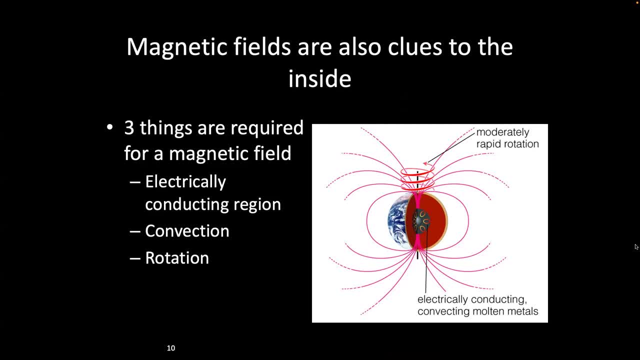 Those are easy to mix up. Jupiter rotates at about 10 hours, So it's very quickly, quickly rotating, And it has one of the largest magnetic fields in the source. Okay, Yeah, Its core is: it's not like lightning. 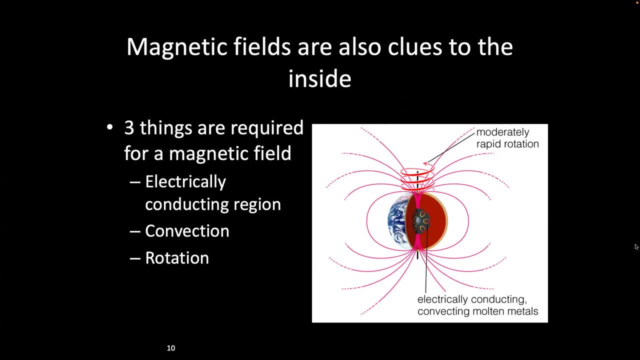 Right. So you said the word metallic. What does that mean? Right, And it's also able to Right, Because metals are what electrically conduct. If I stand outside with this rod and it's lightning, it's about to attack, right? 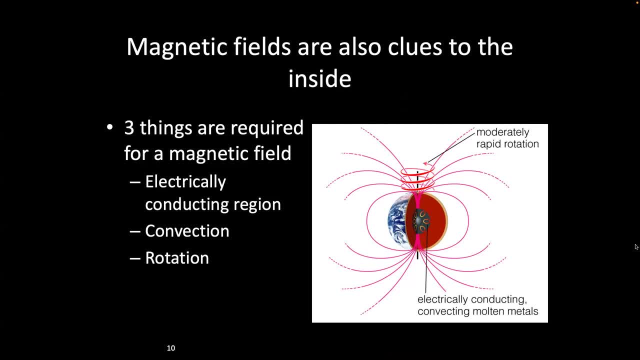 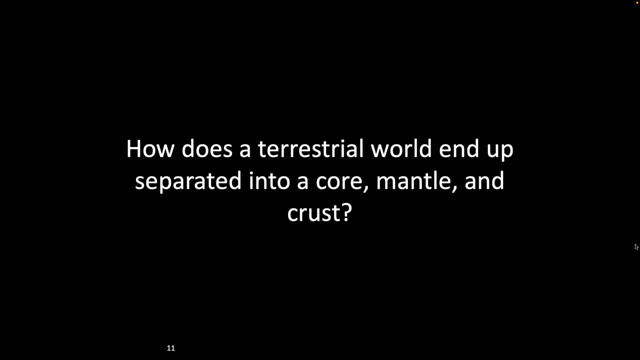 Right, Right, Yeah, Okay. So how does a terrestrial world end up separated into these different parts: A core, a mantle and a crust? Yeah, When it's a hot liquid, it separates. And what's the process that we're separating by? 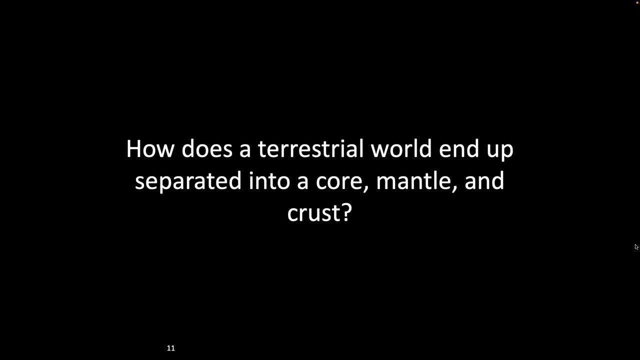 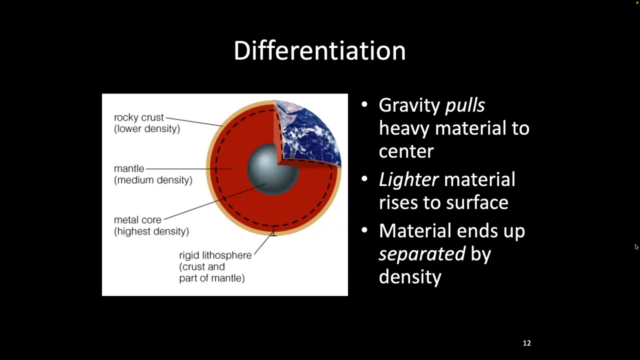 Differentiation And, in Lagann's terms, Yes, Simple, simple talk. Heavy go down. Heavy go down, light go up. Okay, Differentiation is in fact, the right word. Gravity pulls the heavy material to the center. Lighter material rises to the surface. 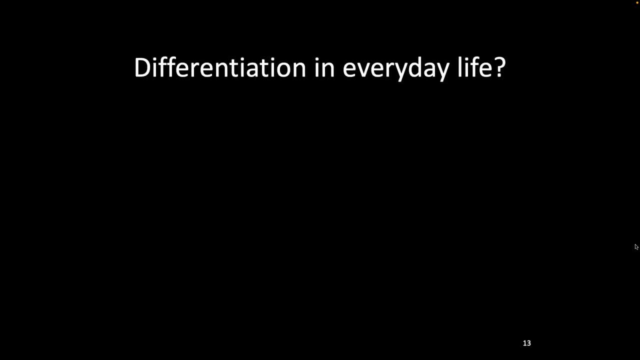 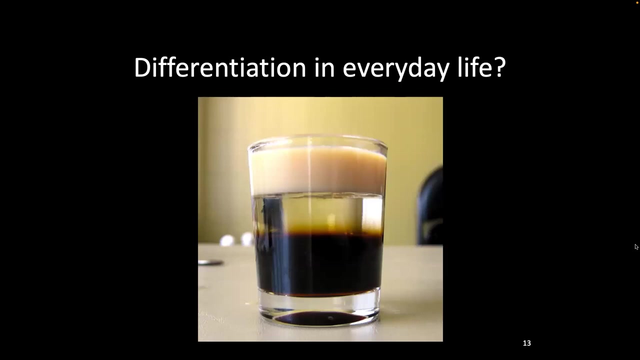 And it separates like this: Okay Yeah, Examples in everyday life: Mm-hmm. Yeah, this is three types of cocktails. so this is, I think, like the clue is on the bottom or something, and then there's like vodka and then cream and they're separated. 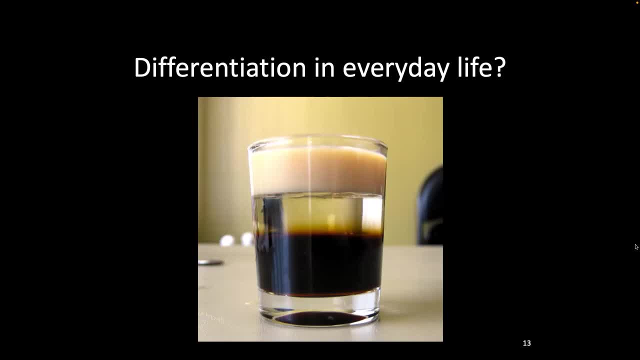 by density, What It's delicious. I mean it's delicious but it's cool, right, and they, or maybe I'll show you a video of this on the next one, You can make like a black and tan where you put Guinness. I'll figure this out next week. 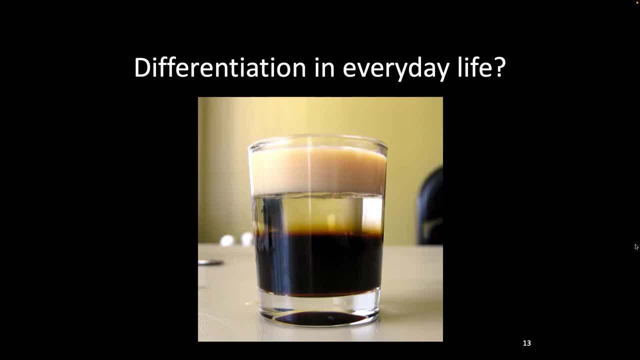 I'll show you some drinks that you can make at home that have these cool separations in density. Future lab- What's that? Oh yeah, future lab. just get 17 beers and then, well, I gotta get rid of this one. 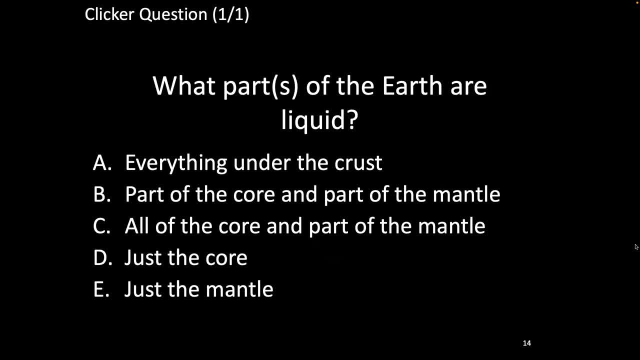 Okay, so what parts of the earth are liquid? Did A- everything under the crust, B- part of the core and the mantle. C- all of the core and part of the mantle. D- just the core or E- just the mantle? 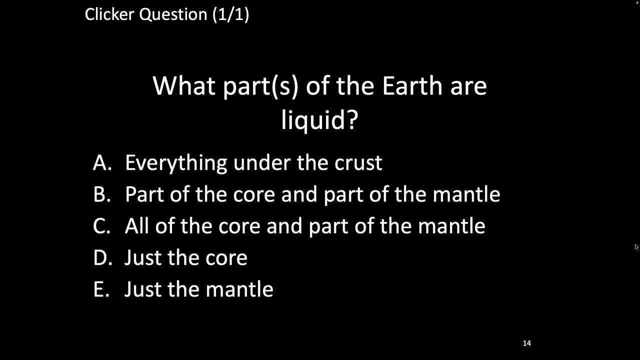 This is something you'll know from your reading, because I know you're all doing your reading right for the next week. Oh okay, What I wrote that one? Oh okay, that's the right answer. That's the right answer. 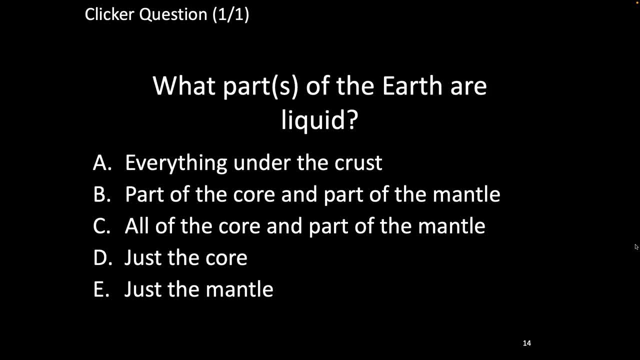 I was ahead and then I forgot. Okay, Okay, Okay, Okay, Okay, There you go. Let me know when you're ready to vote. Vote on three, two, one. Okay, Interesting, All right. So who liked everything under the crust? 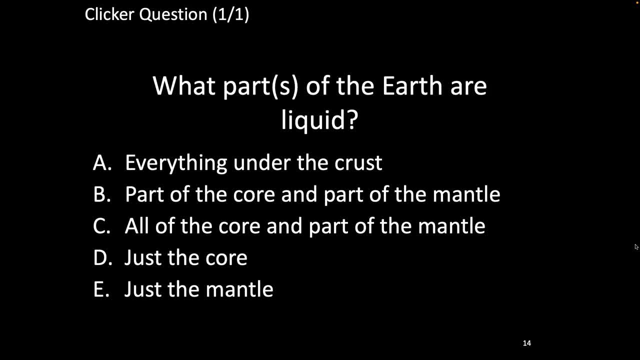 Yeah, why is that? It seems straightforward, right, Yeah, Okay. Who liked part of the core and part of the mantle? Or no one liked it? Anyone like all of the core and part of the mantle? Why is that Okay? What about just the core? 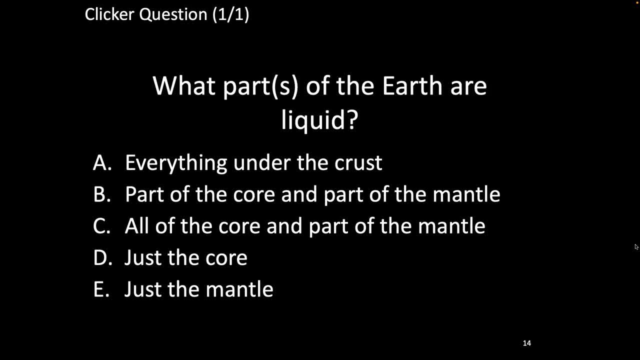 No one liked just the core. What about just the mantle? Yeah, Okay, There's some likers for just the mantle. Why is that? Because the core is the densest part of the planet. Like it wouldn't completely get up there, It would be like fluid. 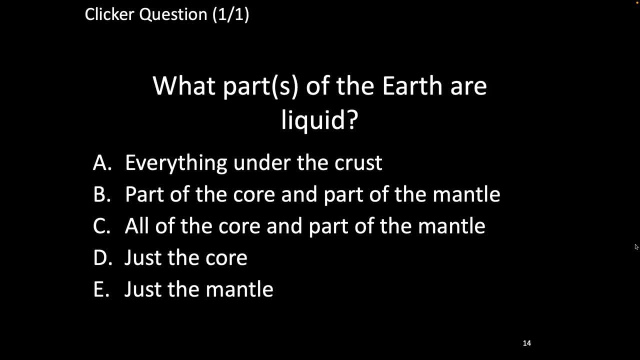 So it has to be solid and dense. Okay, I like that. So we're thinking about like density And liquidity, right? So we're going to get into some weird thoughts, because we don't tend to think about rocks at these temperatures, right? 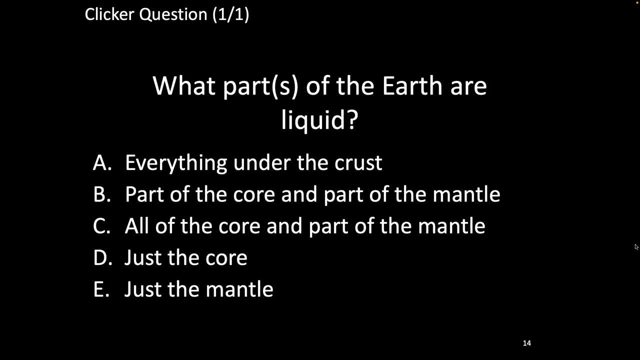 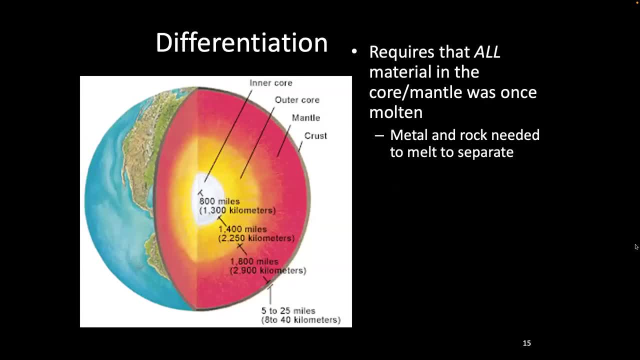 Temperatures and pressures you're about to consider are absolutely enormous And they're counterintuitive. So, in fact, everything under the surface is not liquid. You like that? Okay, So there's a small section we live on, And it goes on. 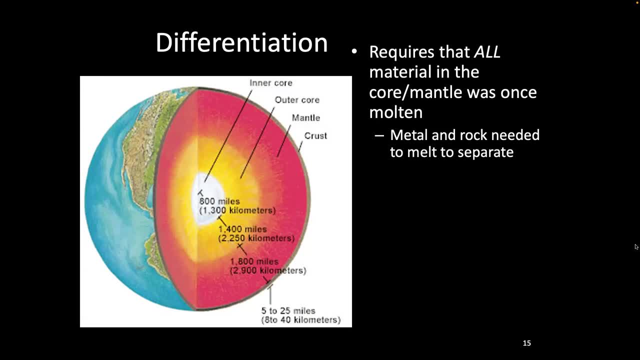 Inner core, outer core, mantle and crust. The inner core is solid, Then it becomes liquid And then it becomes solid. That's not fair. That's cheating Mattel. Okay, So this outer part actually. this should go a little bit to the left. 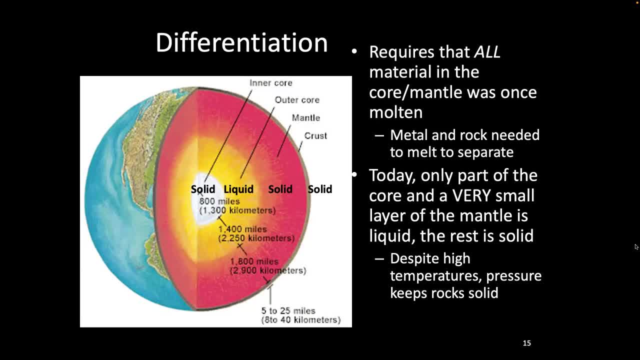 This part here, the outer part of the core, And what you're really having to consider here is a very non-intuitive feeling, which is that at very high pressures, things act solid, Whereas when you're at the right combinations of pressures and temperatures, they will act liquid. 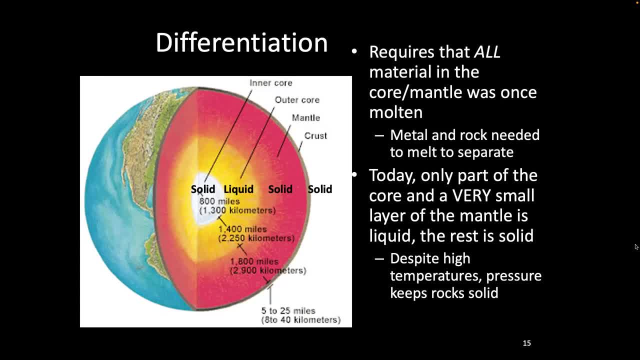 And this is important because in these different regions the motion will be quite different. So, for example, can a rock convect? No, Not, as far as I'm aware, Not once it's in solid form. But when it's under enough pressure for a long enough time it'll act sort of goopy. 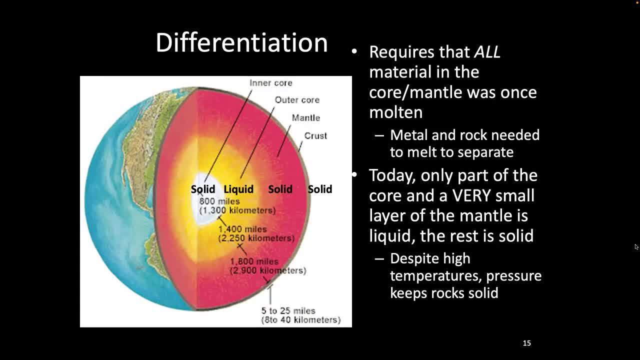 Right. So for example, down here we might have, say, very hot part And the hot wants to get out. So maybe it uses convection in this section And then it uses conduction for the rest of it And we'll talk about. 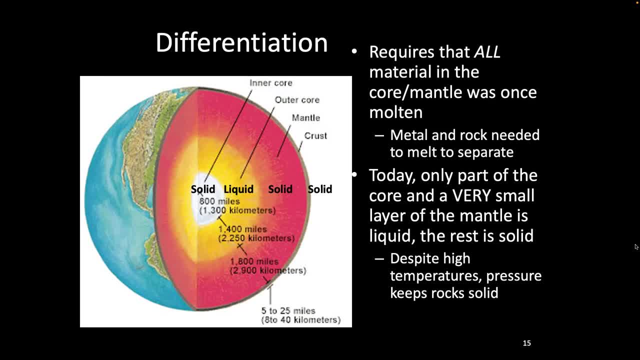 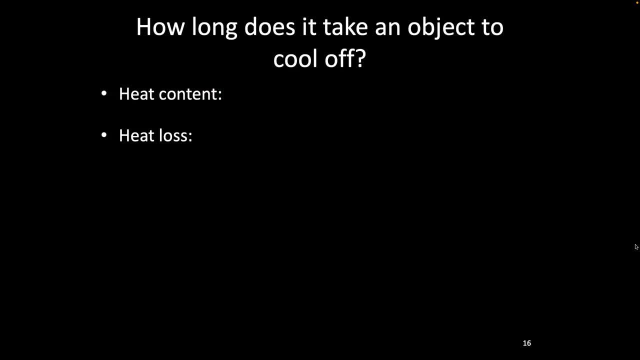 Questions about this. Okay, All right. How long does it take an object to cool off? It depends on how large it is. Good, Anything else. We talked about heat capacity. What does that mean? Cool? It's the ability for something to retain heat. 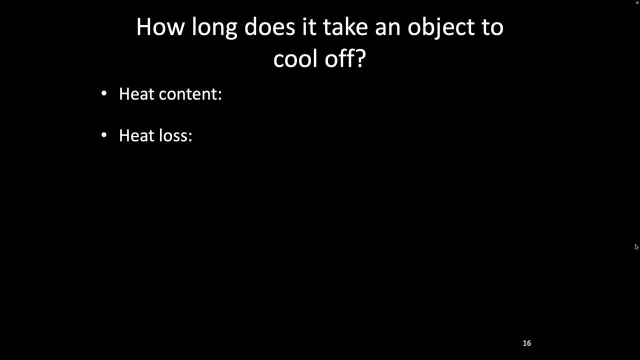 Yeah, that's one thing. So imagine that we have all different objects and different heat capacities. Is there any way? for example, let's say, you make some macaroni and cheese tonight And you get a nice bowl of macaroni and cheese. 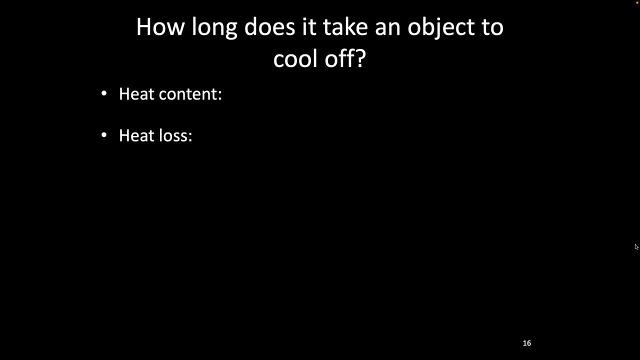 It's really hot. What do you do? Boil it, That's true, But no, Okay, You let it cool down. You heat up the cooling, Put it in the fridge. No, Is there anything I can just do to the macaroni alone? 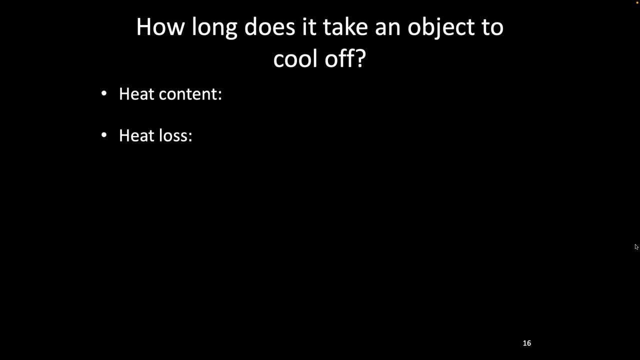 Let's say: I have a spoon, You can stir it. What is stirring? doing How? It's like manual conduction. It's manual conduction. You're letting air in, right, You're increasing the volume, or, sorry, you're increasing the surface area for heat to escape. 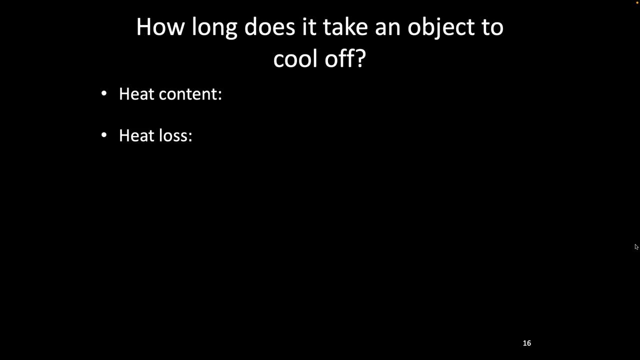 Another thing you can do if you don't want to be sitting there. you can just like make it, dip it in the middle and press the macaroni up against the wall of the bowl. Very weird looking, But it would no. 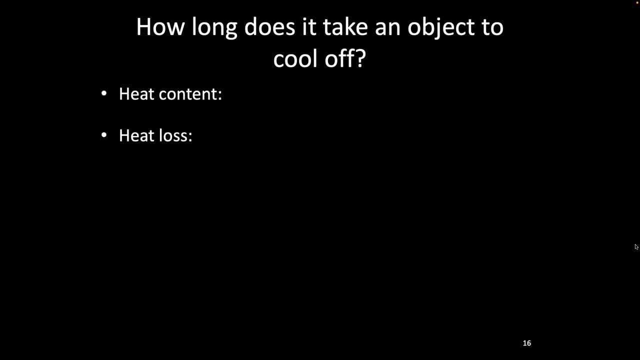 Of course not. I don't make macaroni. But you know what? Eat it warm, Leave it cold. But if you needed to cool something down and increase the surface area, then it'll cool down faster. And in fact, we're going to show this with math. 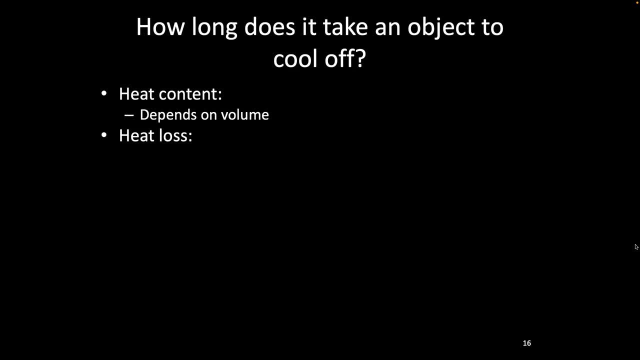 So the heat content depends on the volume. How much heat you have is depending on how much we track. The heat loss is going to depend on the surface area Where you lose it, Right, Okay, If you want to cool something down, okay, you have the heat content and you divide it. 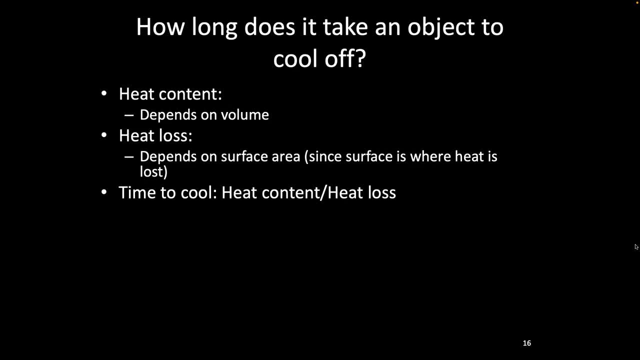 by the loss. How about it? Does that intuitively make sense? Did I pull that out of mind? Let's think about it in terms of my bank account. Okay, So this is all the money that I have, Okay, And this is the rate that I lose it. 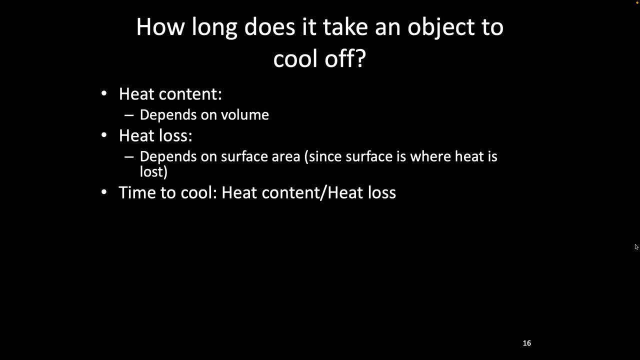 So $15 at $5 a day. How many days do I have Three Right. So the total amount of money that we have in our planet divided by how long we're losing it, for the rate at which we're losing it. 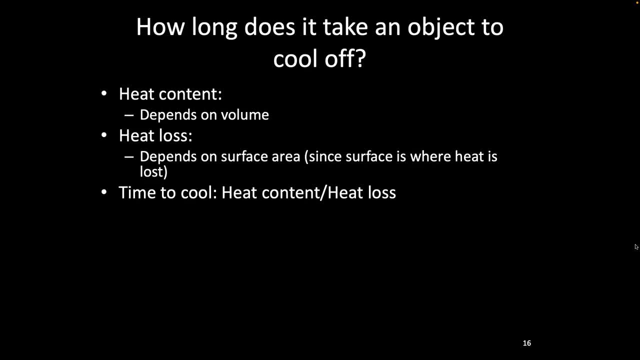 And you can see the units are going to work out there. So this is dollars divided by dollars per second or dollars per year, or however you want to do that, And that's going to end up as a time. Does that make sense intuitively? 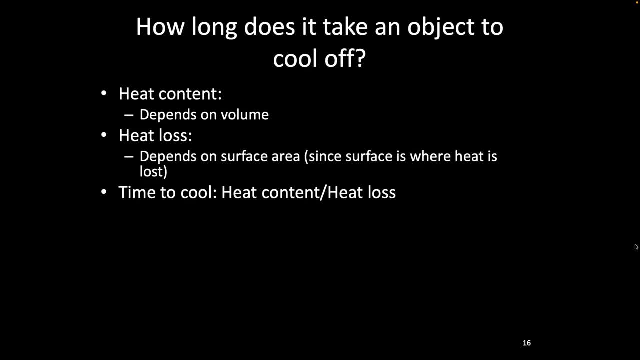 Yeah, Okay. So the heat loss depends on surface area and the volume is the heat content. So what does that mean? that time to cool is going to scale like How is that going to increase or decrease the greatness? You're going to need to write it down. 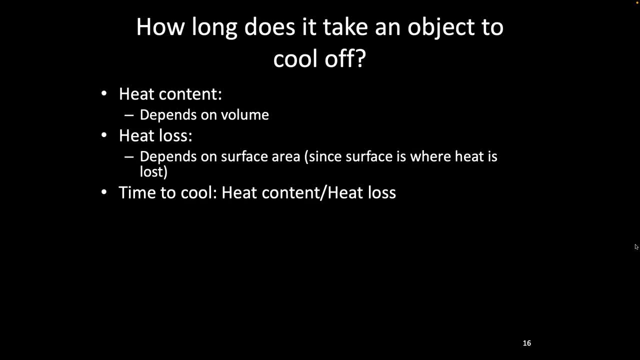 Where's your pen? Where's your paper? One, Okay, Thank God We've got a little stylus. I forgot this one. Cool, I guess It's an awful little pen. I know What was the question, Okay. 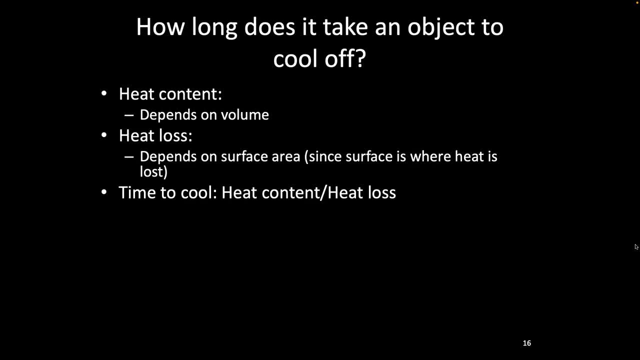 I want you by giving you information. I said heat content depends on volume. Volume depends on the radius. Let's assume that it's a sphere like this. Okay, The heat loss depends on surface area. This is the surface area of a sphere. 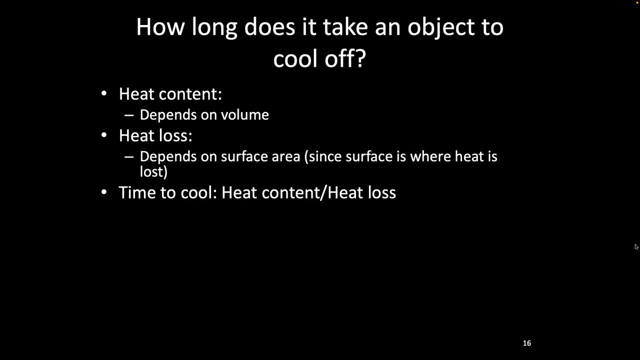 What does the time to cool depend on in terms of radius? Ignore any pi's and 4's and the other ones. Okay, All right, There's a few more. Here we go. This is the one of the three pi's, that is, the jurisdiction of the solar system. 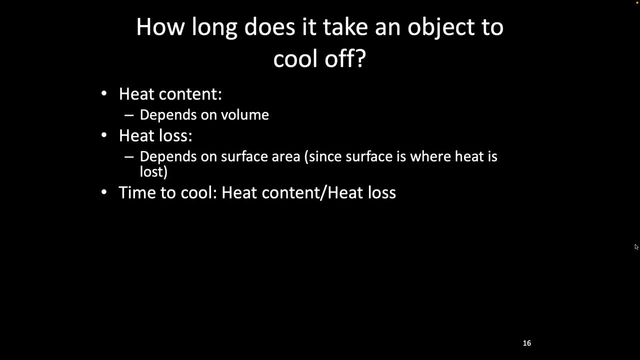 Okay, So does it compare to the rate of increase? Yes, Thank you. Thank you All right, So we've got a lot of news. So one of the key things to consider here is that we need to be careful about the. Yeah. 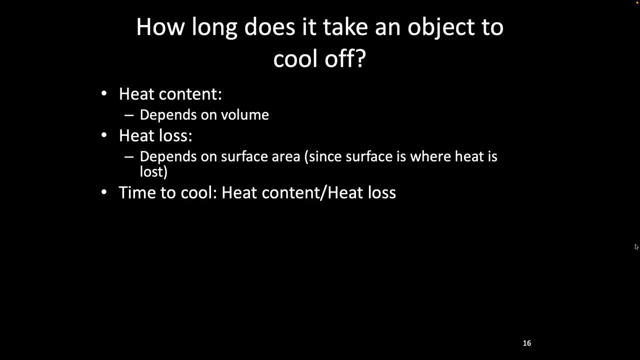 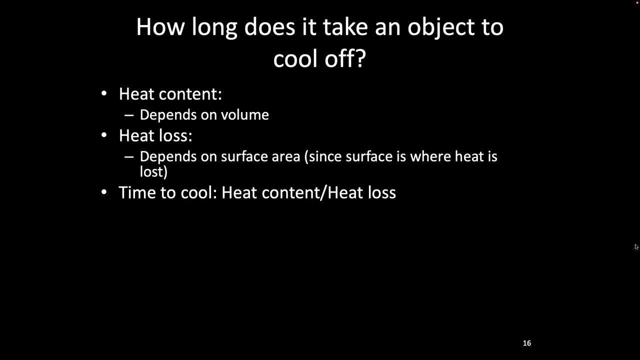 The heat loss depends on the surface area. The surface area is the volume of the radius. The time to cool something down is the ratio of that. What is the time to cool in terms of the radius? So May I ask the same question? 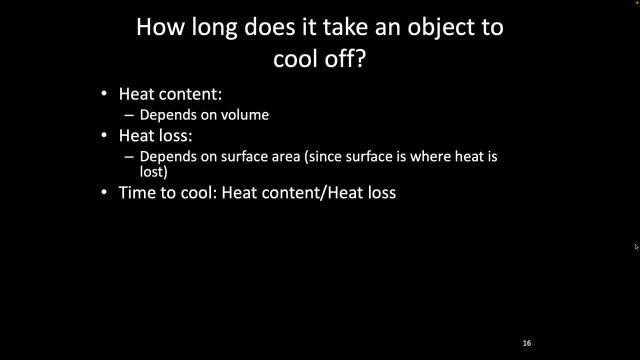 I have a lot of great questions at this point. Positive, Positive, Positive, Positive, Positive. How we doing Two more seconds, two more minutes, Want to ask your friend what they got? Yeah, I actually see that now. 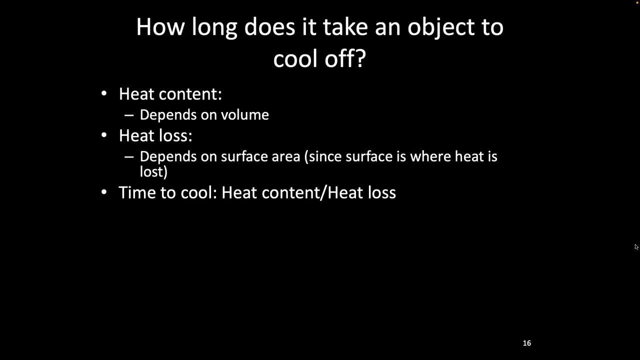 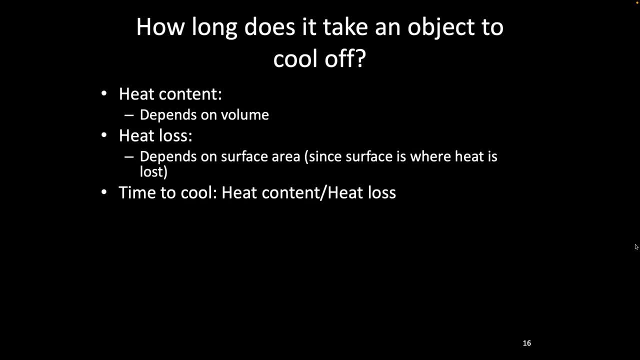 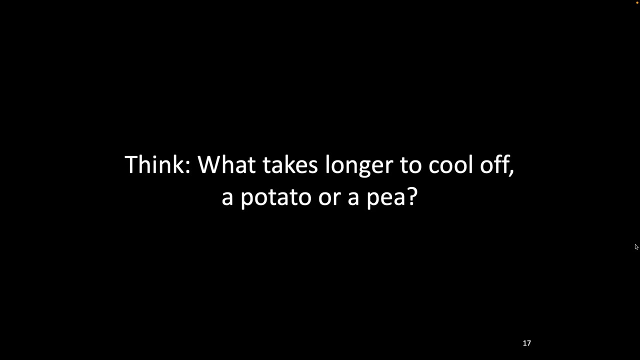 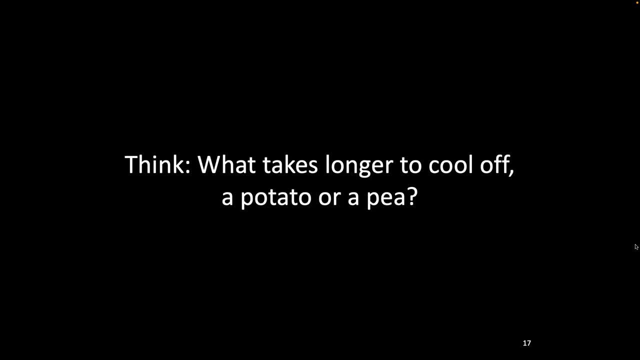 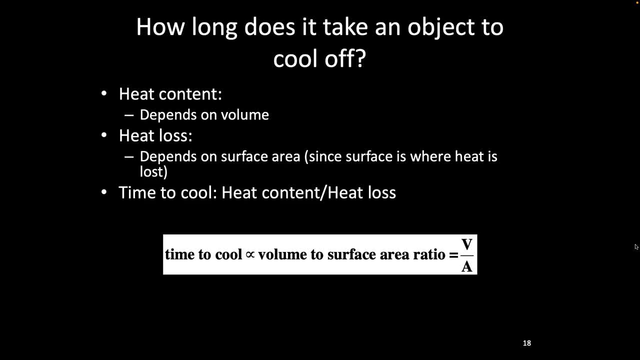 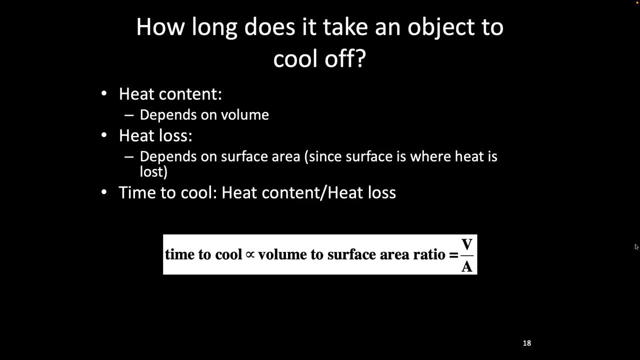 And I'm going to say I don't care about that, And these r squareds are going to cancel with one of those And I just have something that is proportional to r And I'm going to say I don't care about that right. 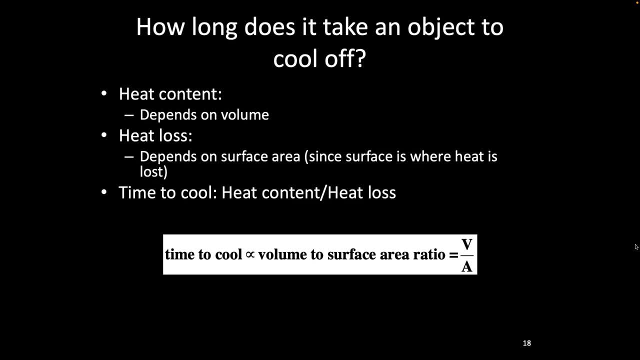 Why doesn't it make sense? The example I followed is like frames. I mean it's important to think about. Yeah Well, I have a lot of this, I'll make a stop. No, I mean in life. So a lot of that. 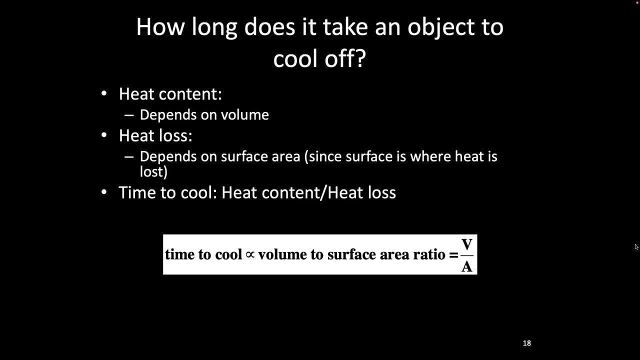 So Out of the value that I have, like, yeah, a longer, longer. Does that make sense? Say that again: Never mind, I'm sorry, OK, we can see. And now I'm just saying, OK, does this make sense? 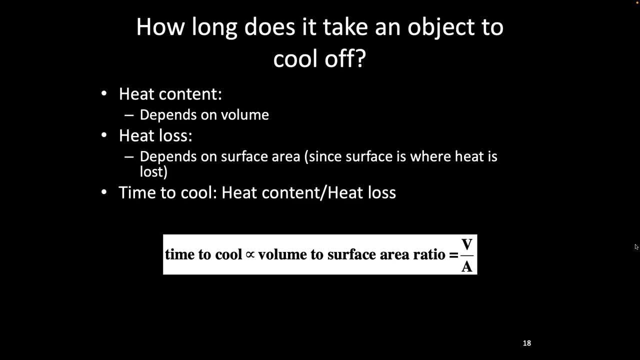 So the potato and the pea is the example, Assuming lots of things are the same, Right. So, for example, if I heated up the potato three hours ago and I just heated up The pea, then obviously the potato is going to cool. but we assume some things right. 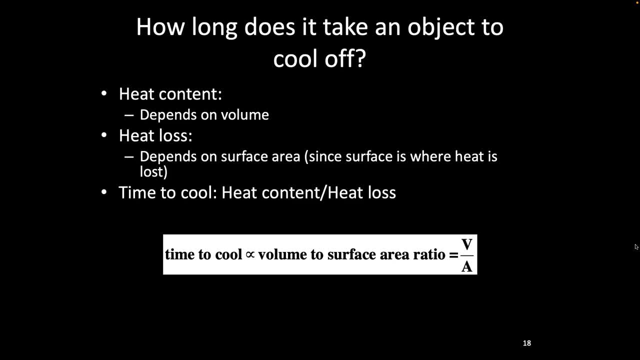 So if you, for example, had two planets the form at the same time, which is going to be hotter? longer, the bigger the bigger one. So I have, in fact, a few planets that we've been talking about, and let's assume that they all form at the same time, even though I've given, you know, evidence for that. 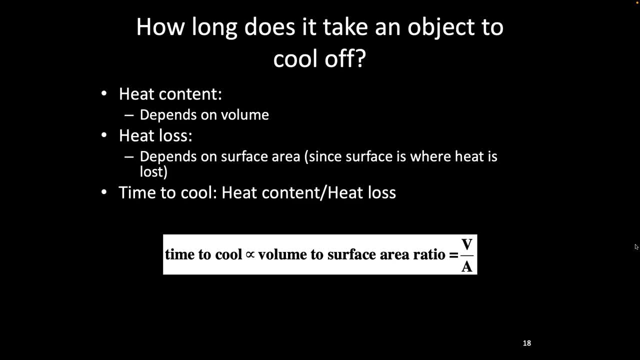 So you have- the biggest would be Earth, And then you have Venus, And then you have Venus, And then you have Mars and Mercury. Which of those is still going to have heat in its interior? That's the biggest I know, And for sure. 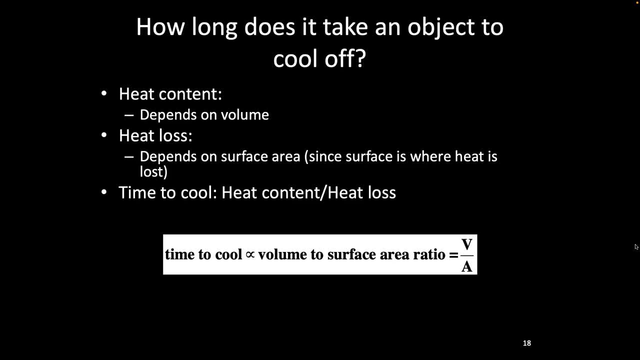 Is that true? We have volcanoes and we're still, like you know, living with a magnetic field that we need, I think, in order to live. Which of those won't? Probably Mercury, Any of them? How big is Mars and Mercury? do you want to know off the top of your head? 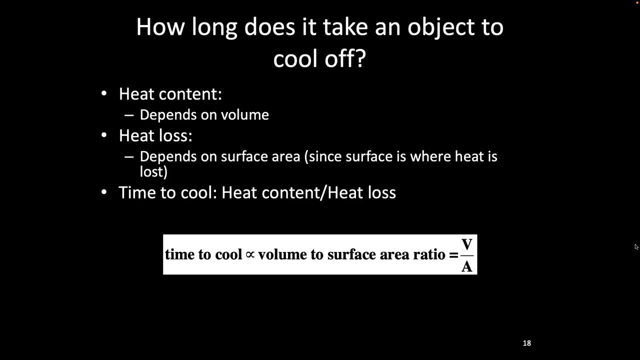 Mars is bigger or smaller, Smaller. Smaller By what fraction? N500? A third. A third in size? How much in mass do you know? That's okay, It won't necessarily matter, But it's smaller. Imagine it's smaller by a third. 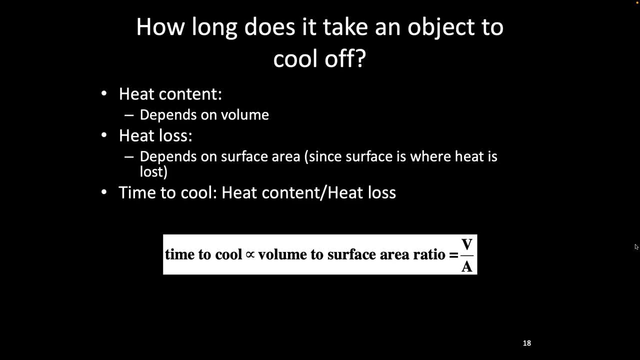 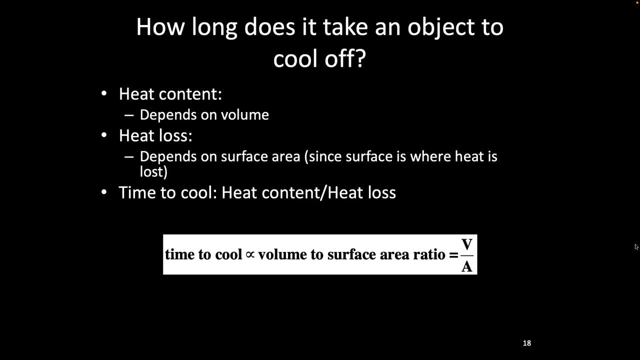 A third, A third. So if Mars cooled off in, say, three billion years, how long does that give us? 9 billion years, And we're about four and a half. Uh oh, It's okay. Okay, Does that make sense? 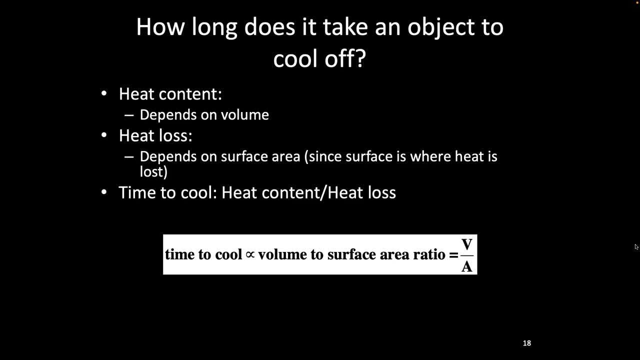 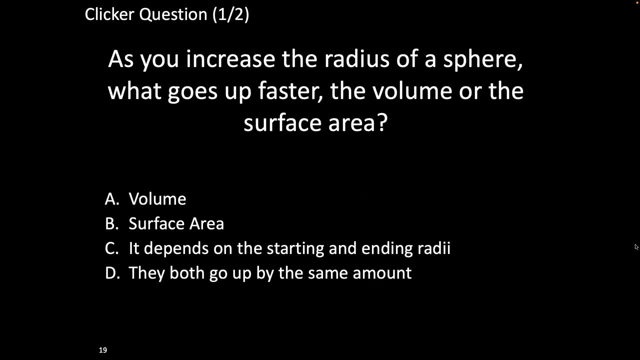 That process make sense, Okay. So, even though it's super confusing and you all hated it, you get it now. Good, That will be on your homework for sure, Okay, As you increase the-. no, that's stupid, Okay. 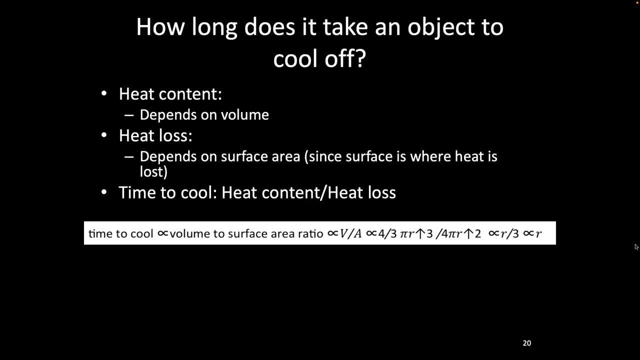 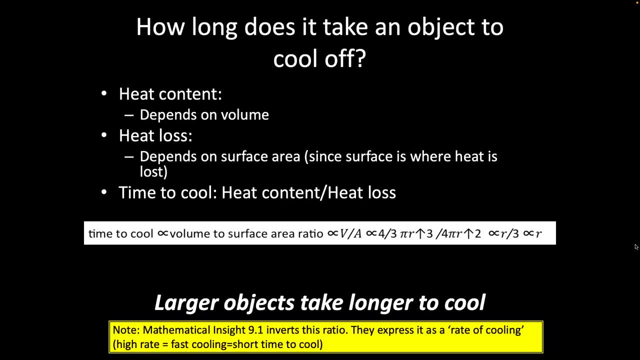 We already did that, Did we do this? Yeah, we did that. So larger objects take longer to cool, right, You can express this as a rate of cooling. So if you just take one over that right, So the cooling rate, what we talked about at the beginning- how quickly does something cool off? 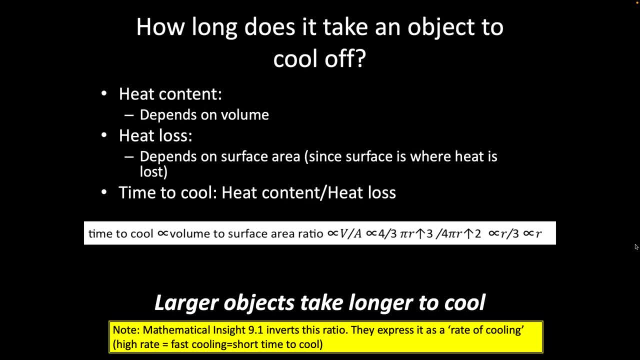 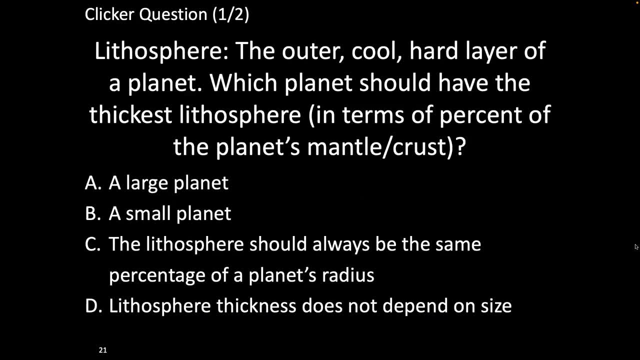 And that'll be one over r, So the smaller things will cool off faster. bigger numbers- Okay, Let's use this again. I don't know if everyone hates it. Lithosphere- what's that again? The outer cool hard layer of a planet. 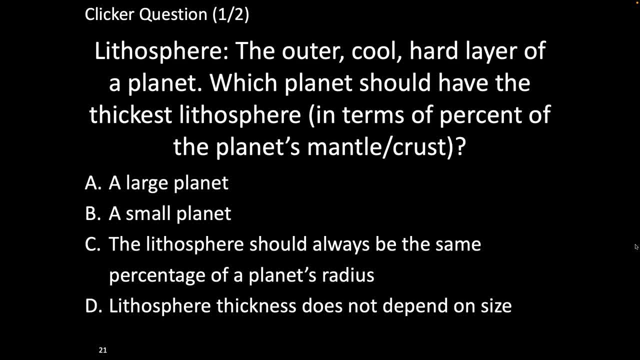 The outer, cool, hard layer of a planet. Which planet should have the thickest lithosphere in terms of percent of the planet's mantle and crust? Is it A, a large planet B? a small planet C? the lithosphere should always be the same percentage. 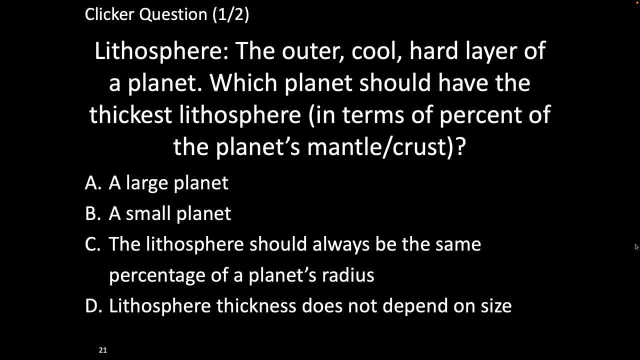 of a planet's radius D, the lithosphere's thickness. Lithosphere's thickness does not depend on size D. the lithosphere's length is the same as the depth of the planet. It depends on the temperature of it. Now let me know when you're ready. 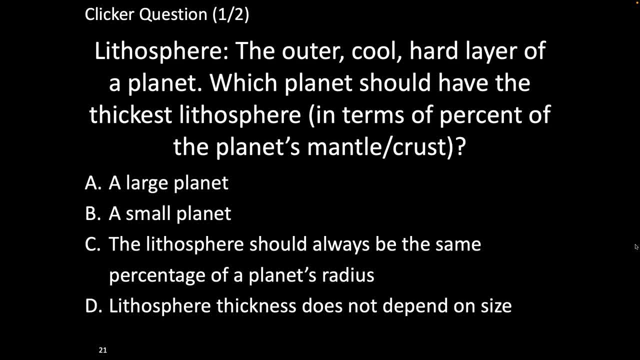 Okay, We'll put it on three, two, one In the back, Slow thinking, Okay, Well, there's enough variety here. I certainly see a lot of threes, twos and fours. A one, That's all of the choices. 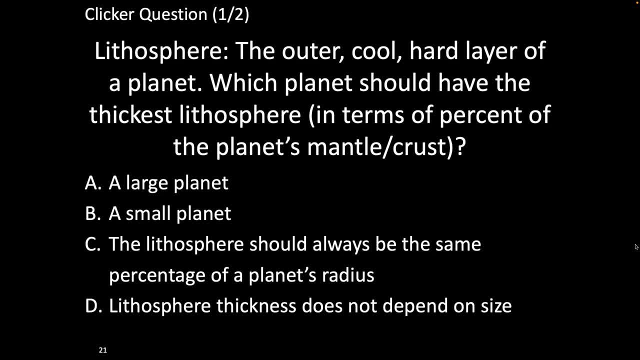 Can you find someone who doesn't have your answer so we can convince them of it? I don't think so All right, let's bring it in folks Who wants to make an explanation here Or defend or ask a question about the question? 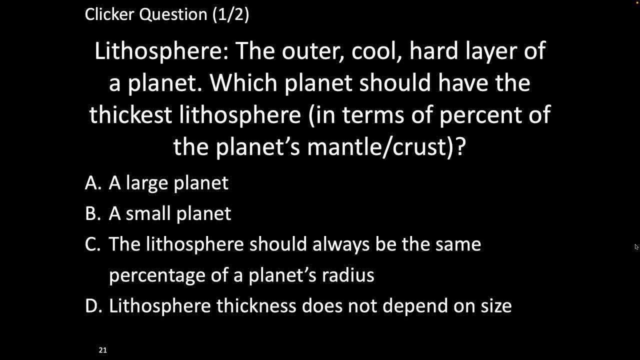 Yeah, let's assume that all things are made of the same stuff. The size is different, Physical size is different, But assume the composition. Anyone like A? So no one fell for A. What about B? Okay, a couple people like B. 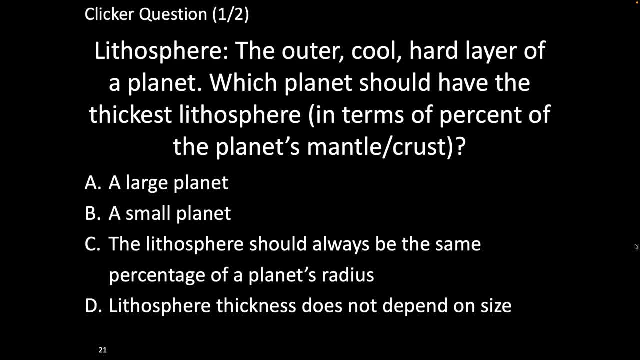 You want to defend B to the class? What about C? Who likes C? No one likes C. Two people kind of like C. Do you want to defend it? People love D, Everyone is for D, Or you just didn't want to answer. 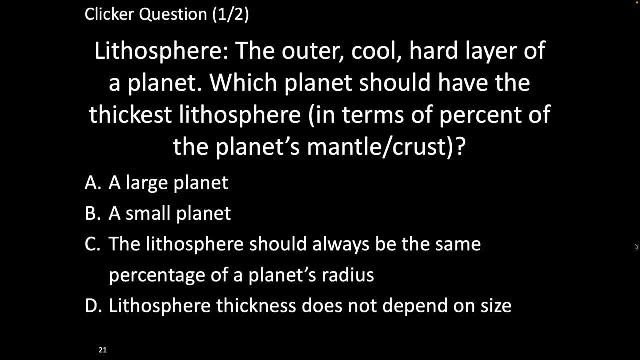 Didn't want to answer. Okay, So let's think about what's going on here. So I said something along the lines of the lithosphere is the cool hard layer of a planet, And then I said some other stuff earlier about how cooling and heat are related. 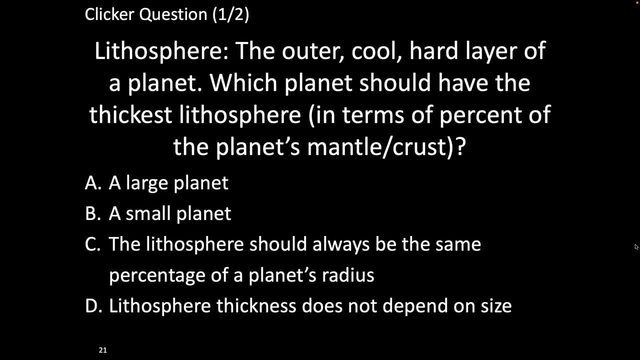 Right. So we have to use both of those concepts together. So here the time to cool is proportional to the radius Right, The stuff that's very, very cold is the stuff that is warm. So the pea was cold, The potato was not. 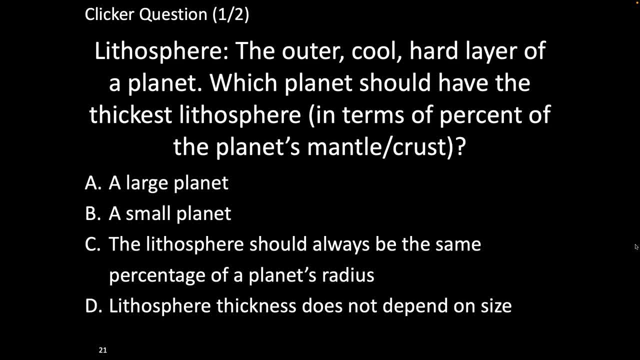 Yes, So we're going to assume two things. We're going to assume all the planets are warmed up at the same time- Just came out of the oven, Okay. And we're going to assume they're all the same type of planet. 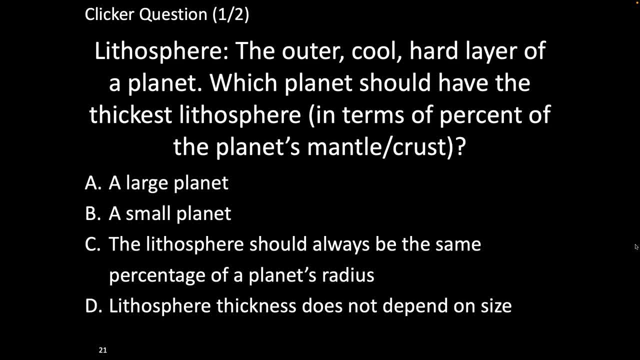 So the potato and the pea are the same density, it's just smaller. Okay, That's the assumption. Does that help anyone? No, Everyone still hates it. Two Why two? There'd be more cool stuff. Does that make sense? 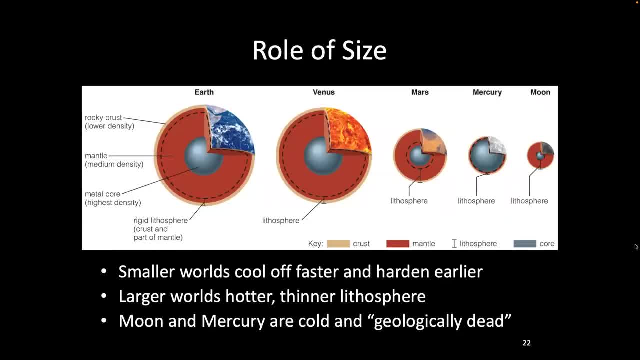 Let's look at these really quickly. In fact, these are the differing planets that we're talking about, And the lithosphere is shown here. Okay, So Earth and Venus. you'll see, this is the side. They're pretty close to each other. 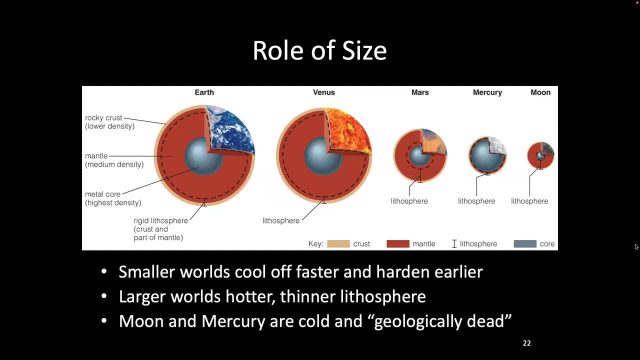 So Venus is our nearest neighbor. A lot of people, I think, think of Mars as very similar in size, but it's not. Mars is really small compared to us, Right? So the Earth's radius is, I think, something like 5,000 or 6,000 kilometers. 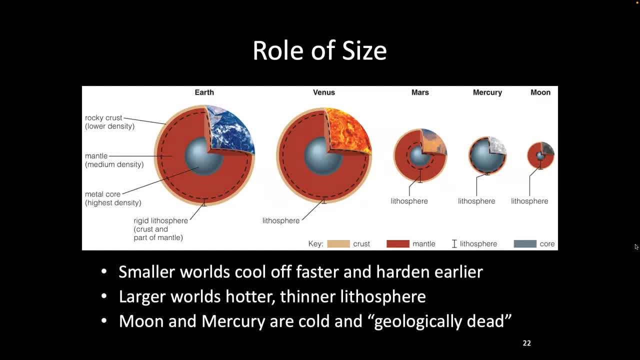 And Mars' radius is like 3,400,, 3,500, something like that. Okay, And look at the size of the lithosphere: It's huge. What about this one? Well, this is the edge of the lithosphere. 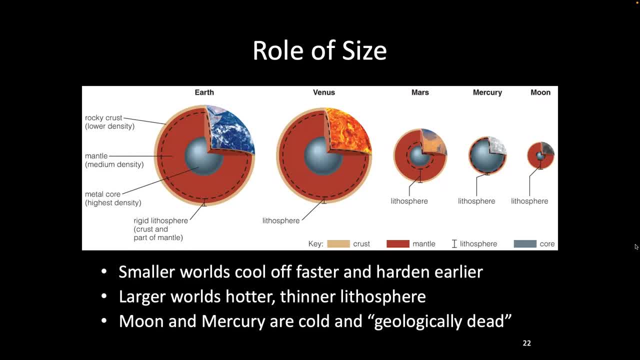 Oh, there, it is Perfect. Sorry, But it's kind of weird. right, This one maybe don't look at that one. That's Mercury. Something weird happened there, Because it's all core. What, Okay? What about the Moon? 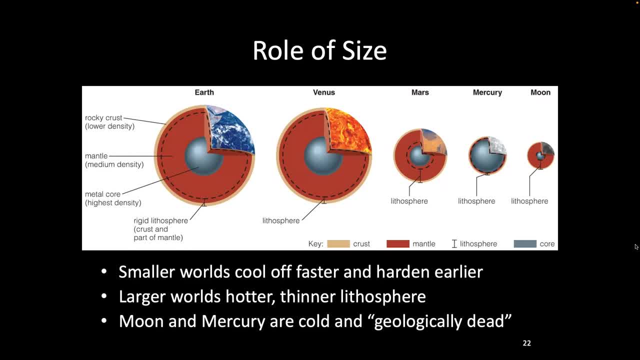 The Moon's the best idea. Right, Moon's are the smallest. Look at the size of the lithosphere. It's massive, Right, Because the Moon's fully connected to the Earth. It's massive, It's massive, It's massive. 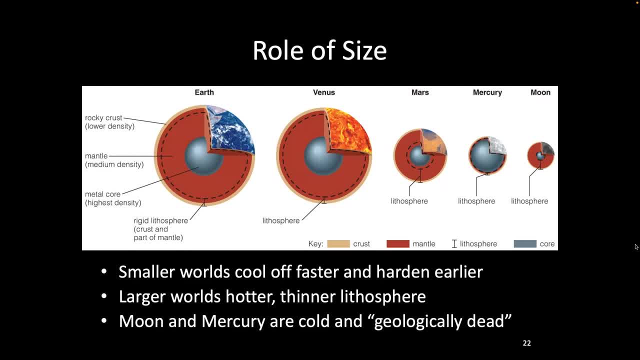 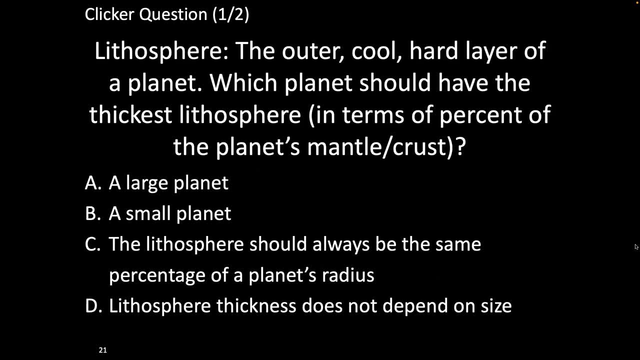 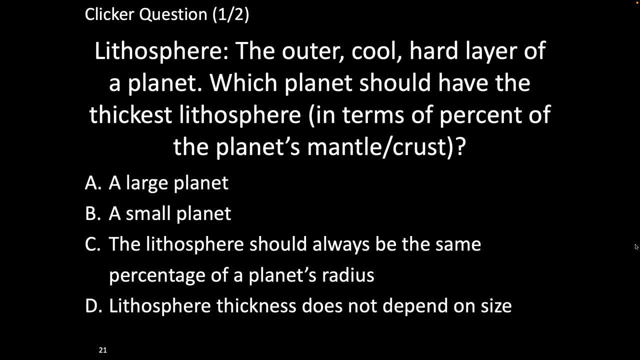 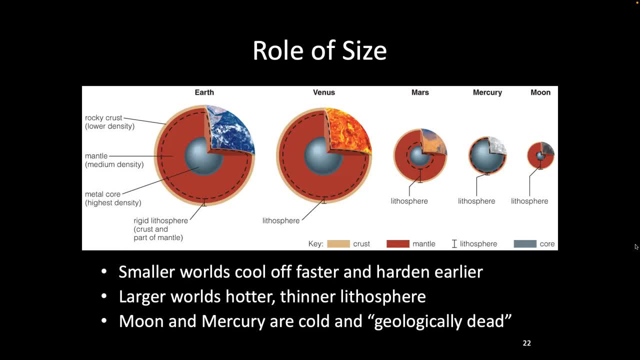 It's fully rocked and it's fully cold right- And that is, by definition, the Moon- all the way until you get to that hard iron core. There is no mantle in the Moon's core Right, So it's deep. 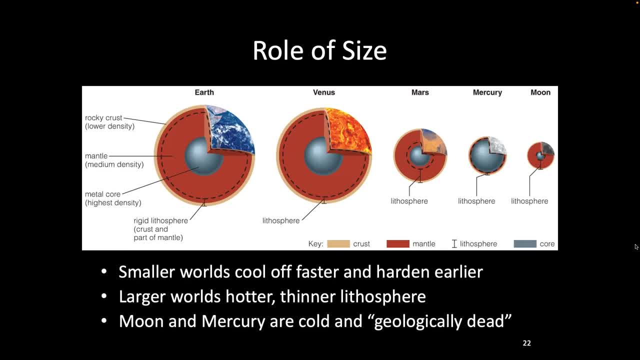 The small planet has a large lithosphere, But that leads us to a really big problem. What happened here? Mercury? Yeah, what happened to Mercury? It's dead. Yeah, it's definitely dead. It has a lot of metal. Yeah, it has a lot of metal. 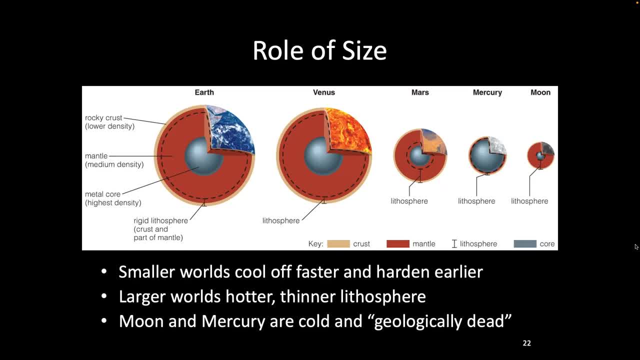 What happened to its mantle? It got hit too much. Yeah, That's probably what's ending up. We're going to when it comes out. we'll talk about formation a little bit later- But in fact we probably think that it had a mantle and that mantle was ripped off. 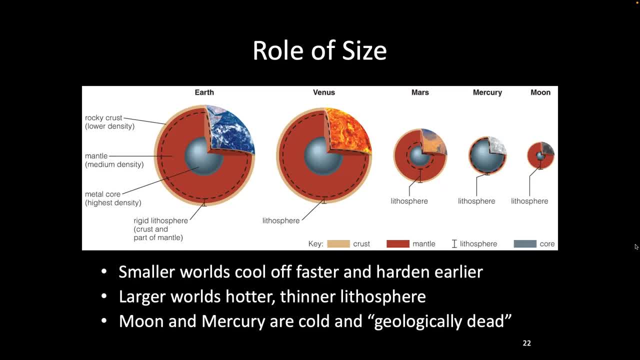 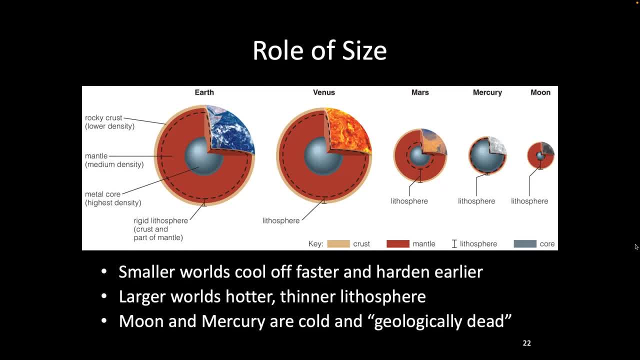 And all that's left is the moon core. Oh, wow, Right, It's kind of crazy. So… It was fully differentiated. yeah, yeah, it's too close. if you're living, if you're living around mercury and you're not on mercury anymore, you're dead. okay, you're going in the sun. people look for what are called um. 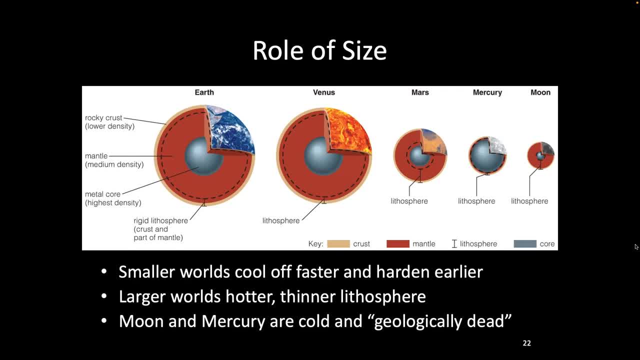 what they call inter-mercurial asteroid, that that lives in between mercury and the sun. we've never found it, but there's a lot of reason to believe that there's no way that they exist. you're too small, you're just going to get pulled into the sun. okay, okay, all right. so planets have. 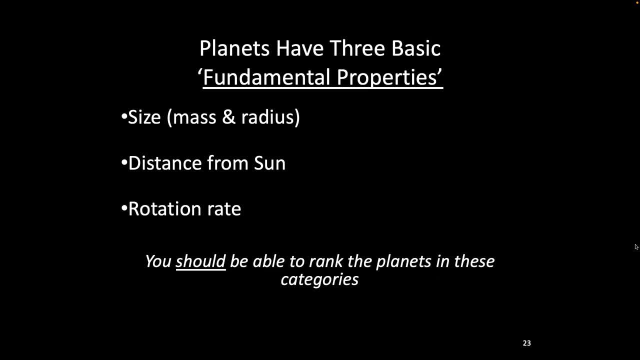 three fundamental properties. okay, size, what does size do? primary gravity: yes, it has gravity, good, what else? okay, what's that larger radius? a larger radius means what about a planet? longer? it's longer to cool. so the interior of a larger planet is good. okay, can we get volcanoes on a planet whose interior is? 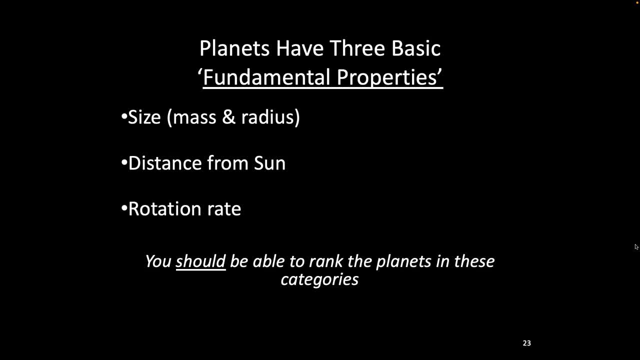 cold? no. can we get tectonics on a planet whose interior is cold? no, okay. so in fact, size of the planet really matters. larger plants will give us more tectonics, more volcanism, until you get large enough that they're not terrestrial planets anymore. they're not rock, right, if they're gas. 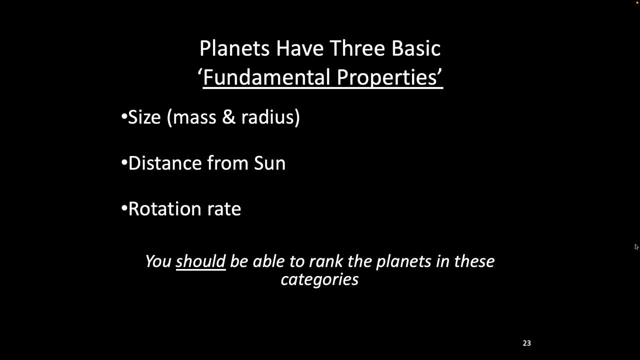 giants, then all this is huge. okay, what about this other one, distance from the planet? did we talk about that at all? mercury, okay, so does the distance to the sun affect the interior of our planet? okay, think about it in this way. we're all having a nice campfire. 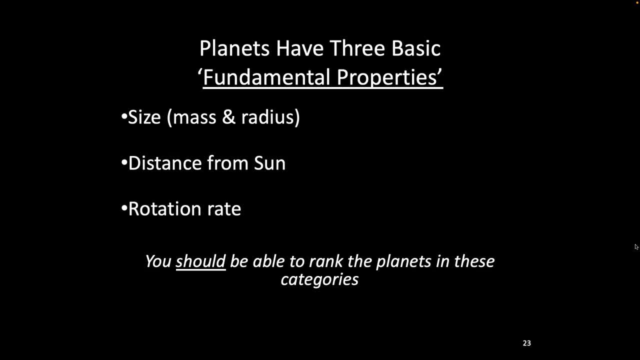 okay, you're really cold. what do you do? you get closer. does that heat your inside? no, not, really not. you get a fever. you die right. so it makes you feel better? yeah, but the exterior skin doesn't actually transmit all the way into things you're here in your body. okay, the same thing is true. 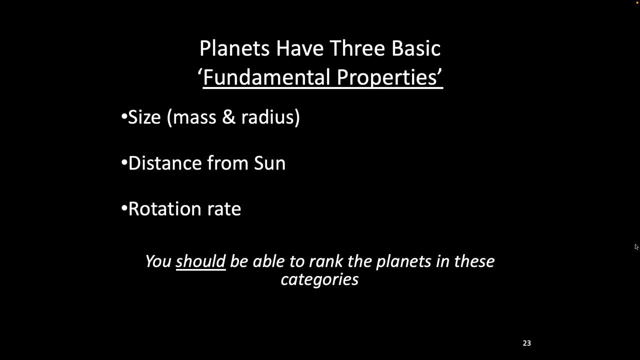 of a plant. we can heat up the exterior a little bit, but we can't put that like. for example, you can't take dead mars and put it next to mercury and then, oh, that's going to that additional solar heating, it's not going to warm up the interior. right, the thing's dead. okay, what about that one? 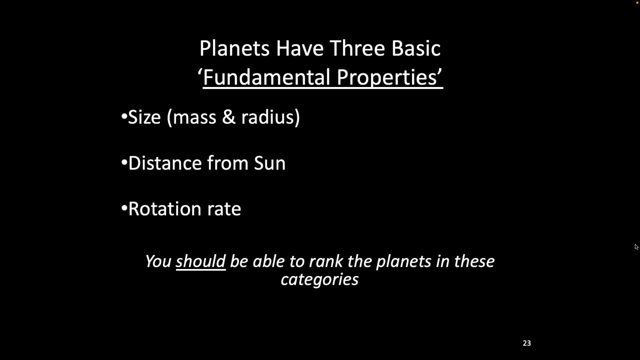 that last thing, rotation rate. what does that matter for? what's that? magnetic field? yeah, exactly, and day and night time, okay, so even cooler, that's true. anything else, doctor had a very brief leave a week ago, so i for you for not remembering more than a week ago. you can ask me. 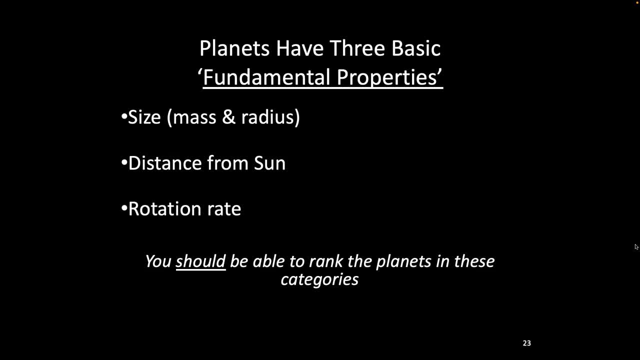 about the seasons, the seasons when something spins more quickly. we talked about something called the coriolis effect, how that turns storms, that makes them more violent, so we didn't talk about it in detail, but we will talk about it. when we talk about after spheres, the end spins really slowly. 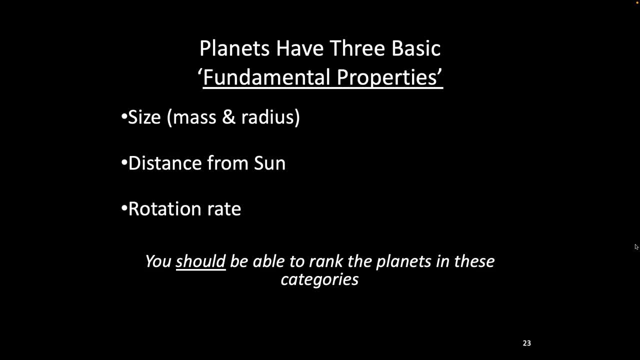 and on the surface the winds on venus are non-existent, totally like still air, okay, whereas if you look at the earth, we rotate relatively rapidly and we have these wonderful things called hurricanes and perennials, and that is from the rotation of the earth. is that weird? what about jupiter? jupiter rotates even faster, and when we see a picture of jupiter, 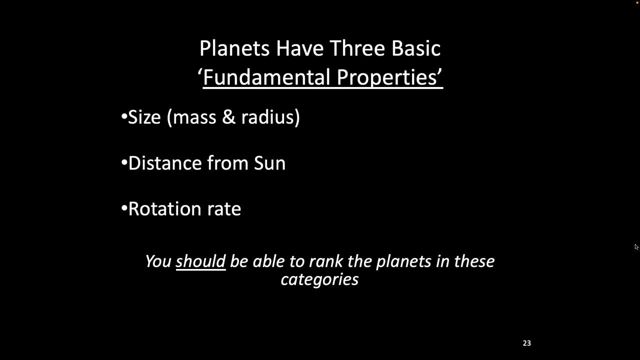 we'll see that all it has is it has no quiescent places on its surface. bison just means black storm. okay, so the these uh planets have three basic fundamental properties- size, distance and rotation rate- and we're going to use these to map them to the things that we can see.